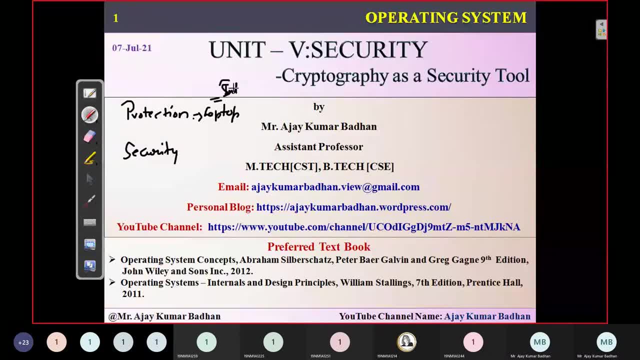 laptop is not connected to a system- I mean, sorry, internet- That laptop is not connected to this particular internet And whatever the data is present in this particular laptop, we need to protect it from what? so? the different type of viruses that may be infecting this particular laptop due to the external sources, something like? you can assume that as something your pen drive Or you people might be in. I mean integrating 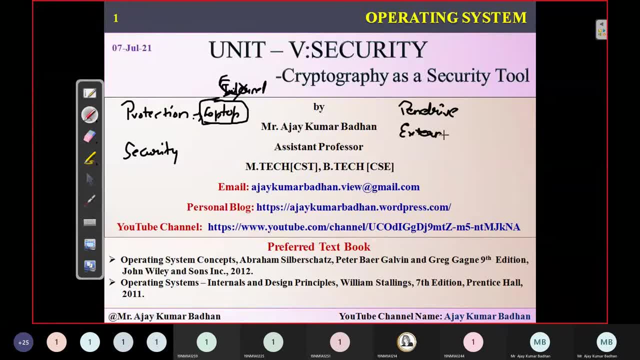 another hardware devices, something like external disk. So these are some of the portable devices, whatever we are having, which we may be connecting to our laptop. So at that time we need to protect the data that is present in this particular laptop. So there is a possibility that this particular pen drive you might have used or integrated this with different, different devices. some, like you, people might have used in your lab And you know that within the lab you might be having virus within your system and that virus will enter in your manager And when you're connecting this to 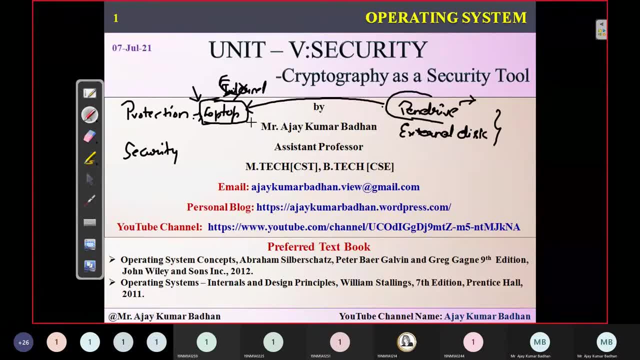 your laptop. you might have laptop- i mean laptop- automatically. so whatever the data is present that will be started corrupting due to the virus. whichever is present in this pen drive, it will automatically will be coming and infecting your system. so we need to protect the data, whatever is present within this particular 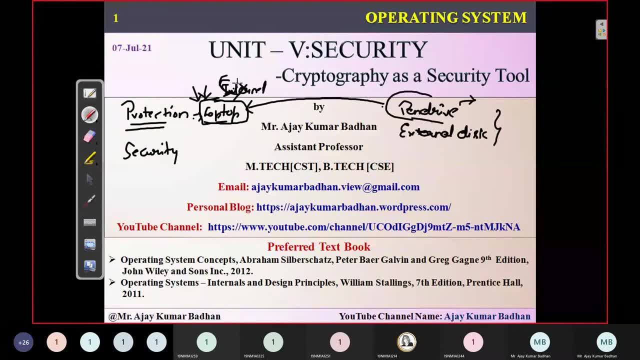 laptop. that is what we call it as protection, and remember that is not connected with the internet connection. internet in the sense, nothing, but there is no attack from the outside network. that's why we are talking about internet here, but if you talk about you, something called a security, what we were. 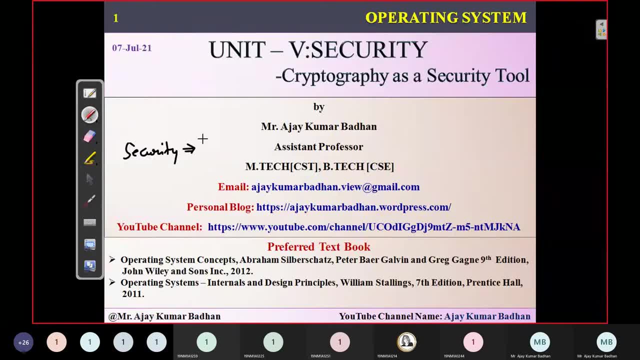 discussing security is something like providing protection with respect to the resources that are present within the system and, at the same time, outside the system. we need to provide outs for security with respect to outside the system. that is nothing, but you people are now getting connected with the help of internet to the outer world. outer world in the sense, nothing but uh. 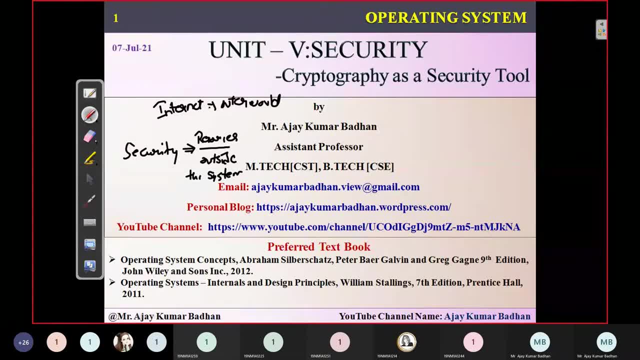 just getting connected to the networks and you people are transmitting the data. so whenever you turn on your mobile data or you people are just connecting a modem to your system- it may be any kind of device, maybe your phone, maybe your laptop or anything different- that means that 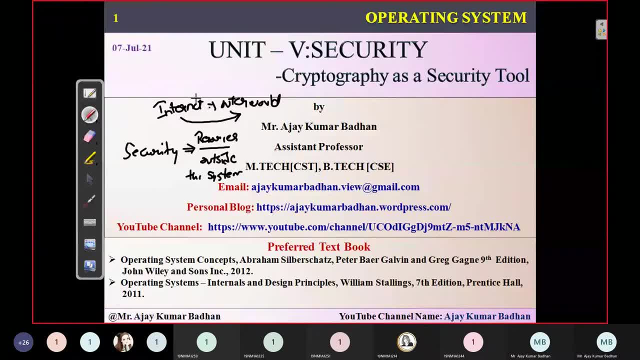 you're totally exposed to the outer world. how, with the help of this particular networks- and we already discussed- every device will have its own ip address. so, using this address, if any other outside the third person knows this particular ip address, he may try to attack on your system using different. 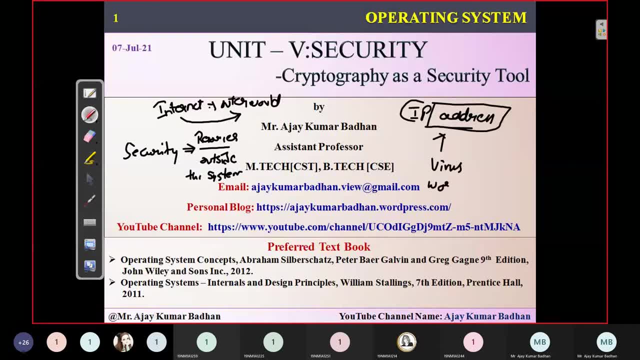 devices. so this is something that we have seen it, something we discussed about virus. we discussed about worms- right, we discussed about other different type of things which can be used in order to attack it- okay, something we call it as trojan horse. so these are some of the attacks. 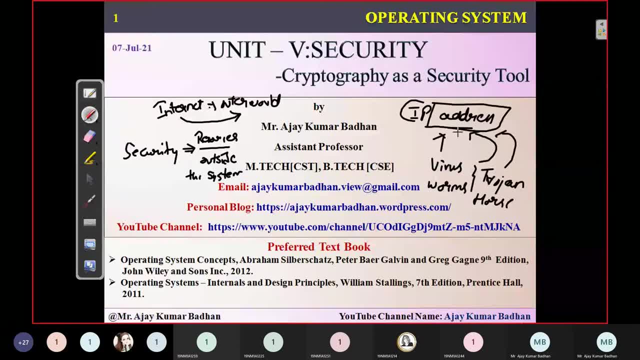 which can be take place via internet. remember that this is via network, not with respect to something called as your pen drive or something like that. for that we are providing security. so now the question is that how we can provide. what are the different tools we have in order to protect the system from whenever it is connected to the 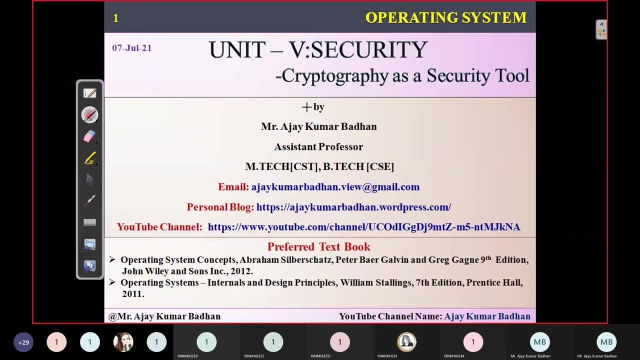 outside world. that is nothing but the networks. so, yeah, the best tool, what we have till date, from the beginning, is something we call it as cryptography. cryptography is the only tool which we are using right from the beginning, so let's go ahead and see what exactly it will consist of. 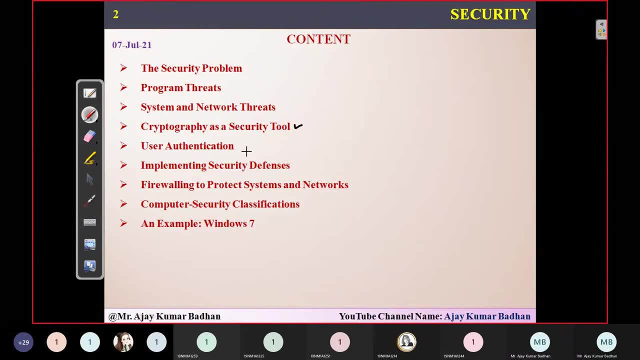 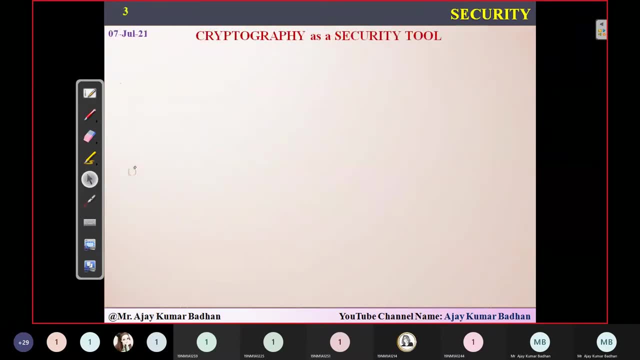 so today we are going to discuss about this, uh, something called as cryptography, as a security tool, and then what are the different things we have with respect to this particular thing? now, if you ask me about security here, in this particular thing, uh, cryptography is the one which 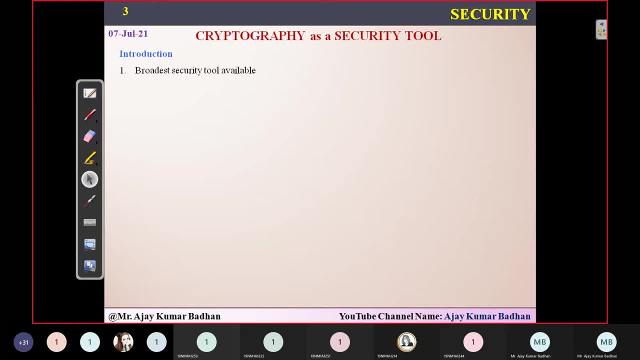 is used. cryptography is actually the one which is used for transmitting the messages and now, as i told you that cryptography is the only tool, we are using it, so we can say this is one of the broadest tool. why it is broadest been. most of the research work has been done on this particular. 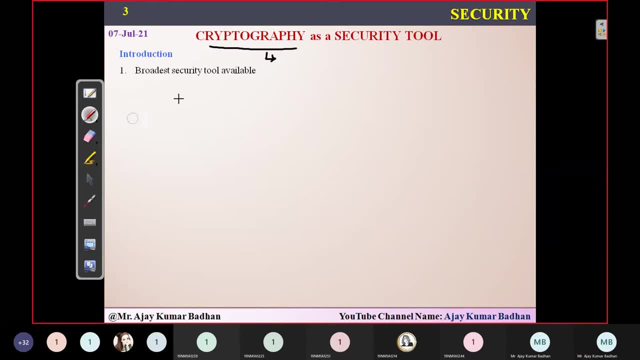 format, whatever the format people are seeing here. all the research work is done on this particular concept called as cryptography. we have, uh, different, different organizations here. we have something called as nist- national institute of standards and technology. we call it as national institute of standard and technology. 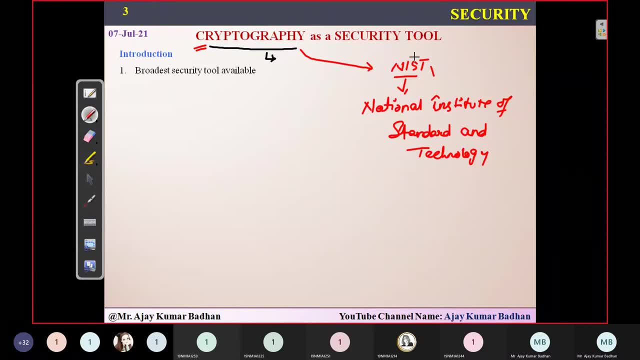 actually has developed this particular cryptography. they are the one who actually develop new, different type of technologies which can be standardized all over the world and which can be used throughout the entire world. so this is one of the organization like this. we have different organizations also, but this is the most popular among all the organizations. 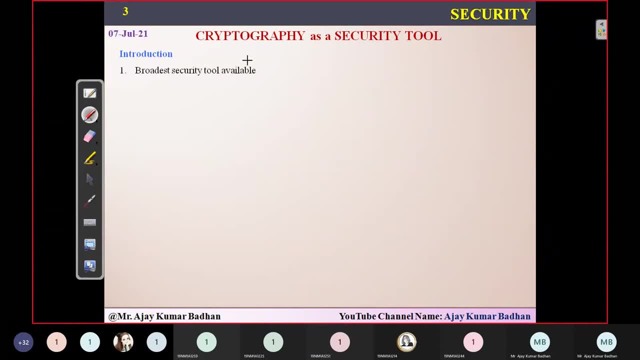 what we are having so here, the tool, what we are talking about here, is nothing but cryptography, and this is one of the broadest tool. what we are exactly having um here, whenever you people are actually transmitted, so what exactly this particular thing, or just particular cryptography, is going to do, is this particular thing is used to send transmissions. okay, it is. 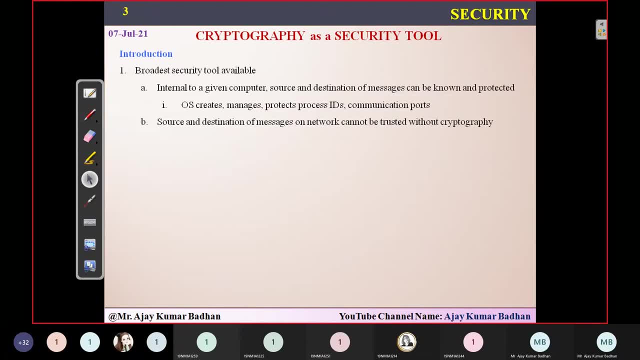 actually used for transmission of data. transmission of data over what? over network? for example, you wanted to send a gmail. you try to send a gmail to your friend, so how you can transmit that particular gmail? definitely, you people have to give something like two address, then you have. 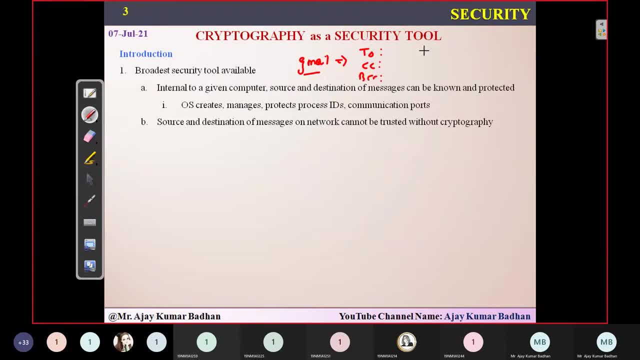 something like cc, bcc, and after that you people have a site, and then you have to send a gmail to subject right, and after that you'll be having some content to write. and then, finally, attachments. if you want to attach any file, you can do it, and once you click on a send button, whatever the data. 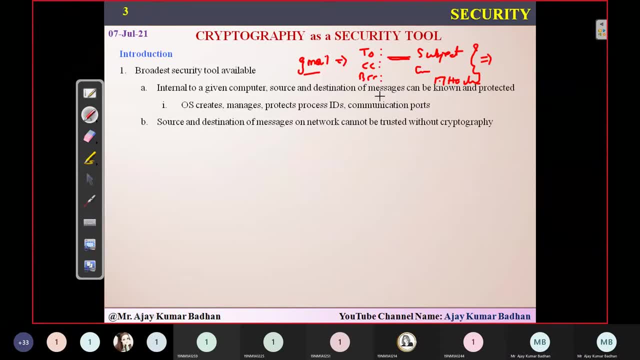 is present in this. it will automatically deliver to the destination address, whichever you're giving, and definitely how it is possible to transmit it. definitely there should be an internet connection. if you don't have an internet connection, is it possible to send a mail or something like that? it's not possible. so that is what he's exactly saying here. so here, in this particular 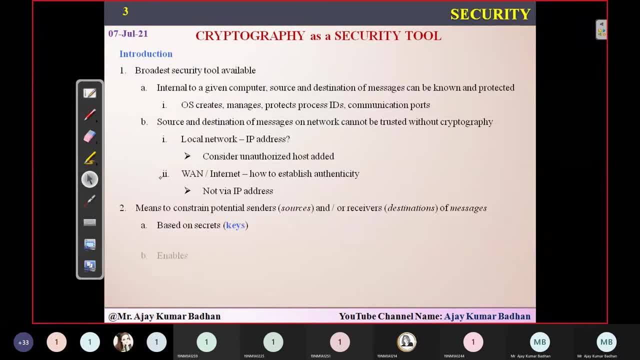 example. uh, let me show you up once. yeah, so here, what he is exactly saying is that, uh, whatever the computer we are having, that will be uh, from where you people are transmitting the data. we will call that as a source and the message will be reaching to your friend system. right, it may be on mobile phone or it can. 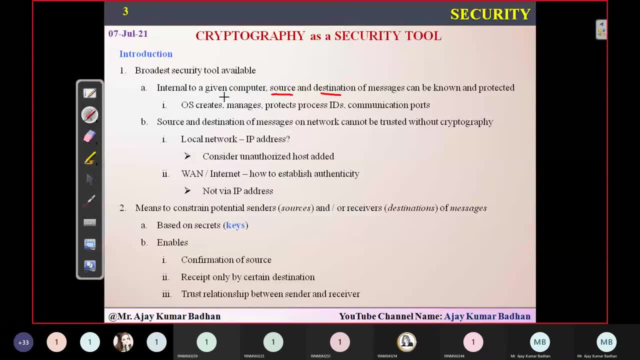 be your laptop. that is what we're calling it as destination now here. whatever the data you're transmitting from one particular dessever computer, i assume that this is a source computer, this is a destination computer. this is a source, this is destination from here. you wanted to transmit some data through here, so definitely. 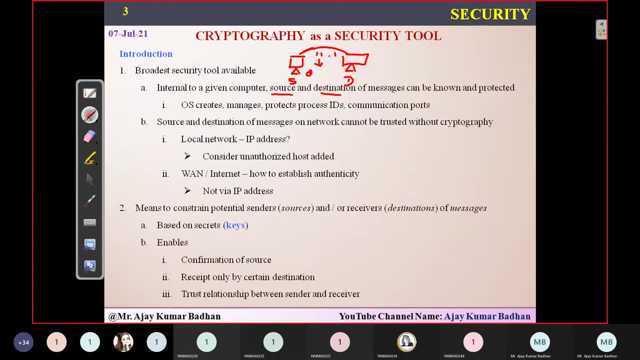 what is this part? this is the one which is we call it as open network. this is what we call it as open network means anyone can try to come in between and they can try to hack the information. what is present, through which we are transmitting the network, because that is an open source- it's. 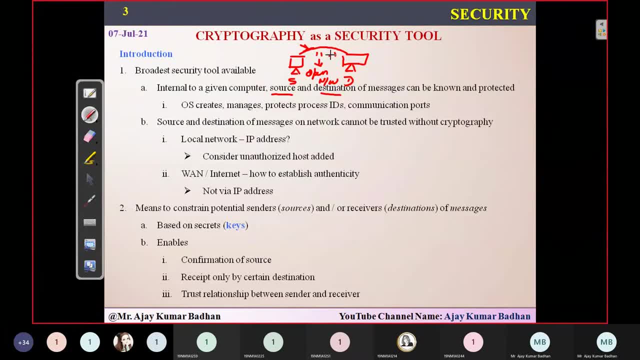 an open network, anyone can come in between. so here, whatever the data you're transmitting, we should make sure that, whatever the information we are transmitting, that is secured, secured and it is securely reaching to the destination. suppose you people are sending hi, how are you? the same message should be transmitted here in a format of the way you are written: hi. 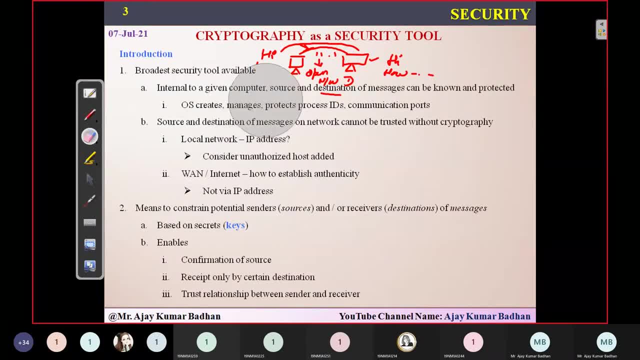 how are you? something like this: okay, so for that purpose we are using cryptography. you know what exactly this cryptography means. here is nothing, but in simple terms, what i can say is suppose, as i told you that i'll be sending a message, hi, how are you right now? let us suppose you people are transmitting this on a whatsapp to your friend. 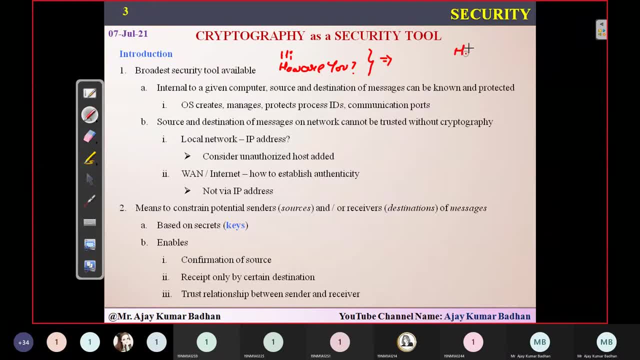 now your destination means whoever the friend is, she will also getting. she will also get the same, or he will also get the same message. hi, how are you fine? that's fine. whatever you're transmitted, that is, only has been delivered to the destination, but in between, where it is traveling in the air. 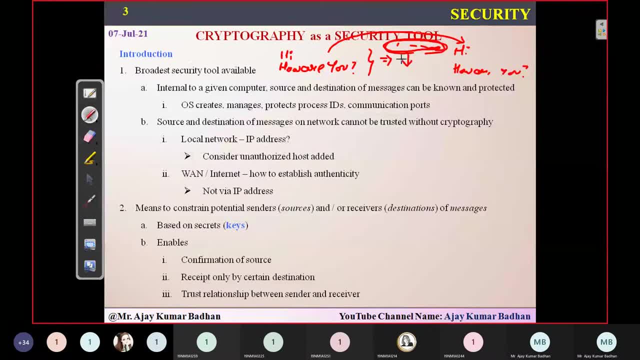 in between. it is traveling in the air in for this purpose. what they're going to do so that the third inbox that we will have to get is to send that message to their destination. so you people would be sending calls to the destination, so you need to text that message and you can see there. 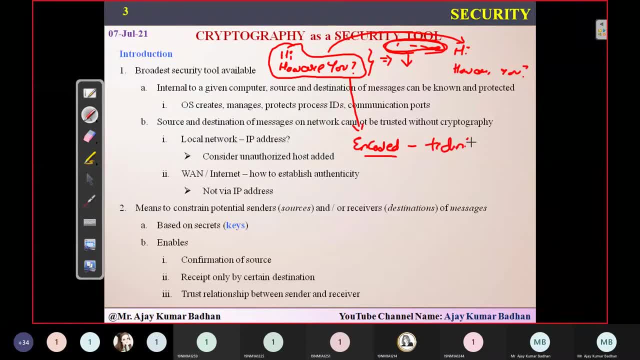 something like that. right, that's showing in there personally you. you will be sending an account letter like: ah, how are you? and here you arerier, uh, nord, can't n your time, sir. you have to check first and then you start sending more or less at your destination platform. so if you are writing that message, i will not vibes so. or in pangolin in my google library, using a word, is that i will not be sending that message. you people are sending the onto your device. device ion is going to send that message to you as soon as that message has been sent and that message. 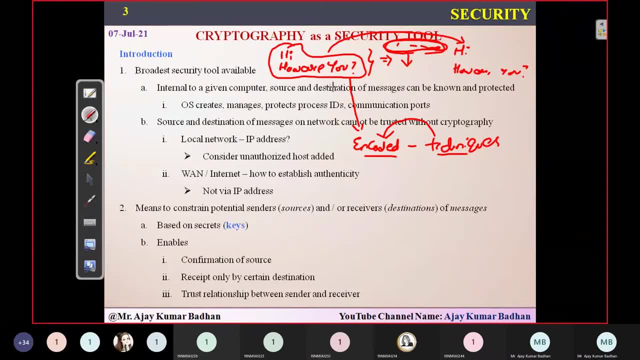 will be sent to you, uh, when you post it to other devices, and after that you can see that the message is presented. so write your email and use it here in the second address of Rahul, which doesέ this message. however, you know that will be something like uh, just a normal, rough estimate. 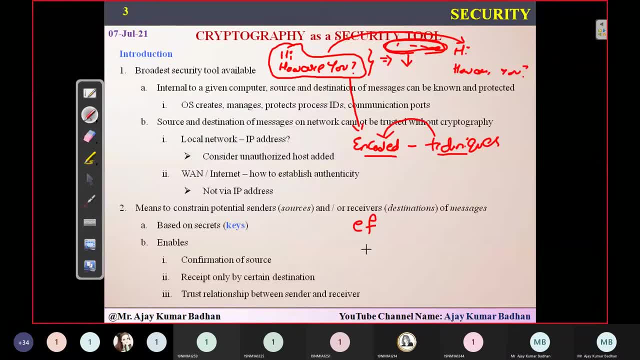 i'm giving here something. it will be like e, f, g, k, h, a, b, c, z, a, k, something like this, even for the question mark also, you will be having something like zero. so this is a message which will be transmitted over the network. can you read this? 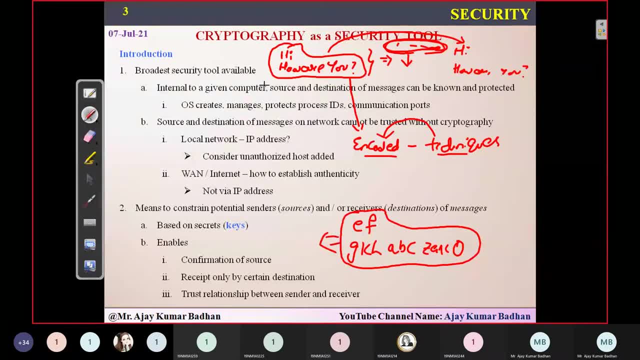 particular code. i mean, read this message. what exactly? this is the same thing what i have written: hi, how are you? this is also hi, how are you? but only difference here is when it is transmitted over the network, it will be encrypted in this particular format. okay, so they will be using some. 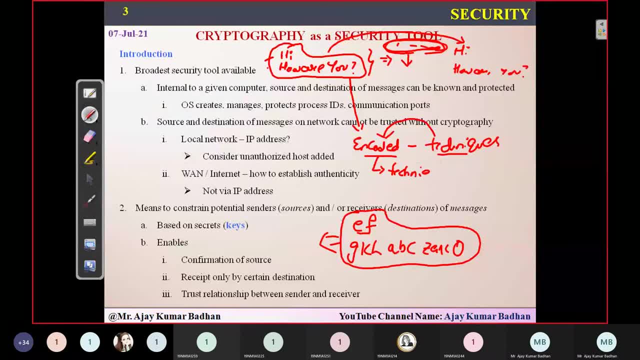 encoding technique here, some encoded technique we are going to use and using that technique, we will be converting that message into this format and, one by one, will be transmitting it so that if a third person try to access information, he will get this information now, since he got this information, he will. 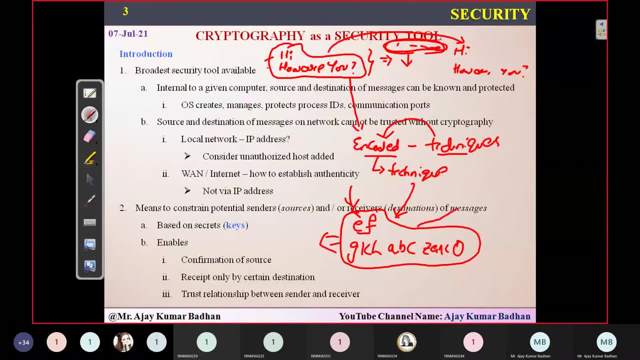 not be able to read the actual message. because to decode again this measure, message has to be decoded. so to decode that message again, we require something called as a term, called as a key. that key is what we call it as a secret key. okay, so if we, if you people, are having this key only 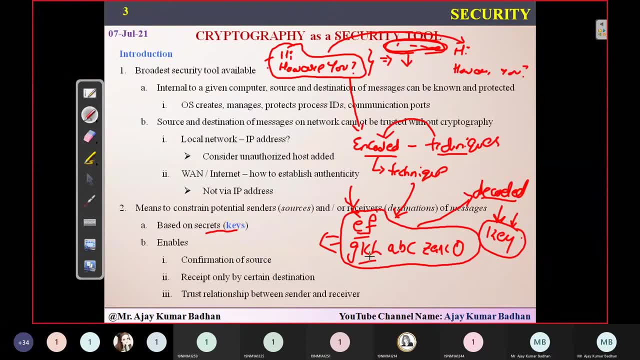 that person can try to uh what we call decode this particular message. one more example what i can do you. the best practical example is your whatsapp. i don't know how many of you open that site and read the message and sayitol: where did you see my message request? 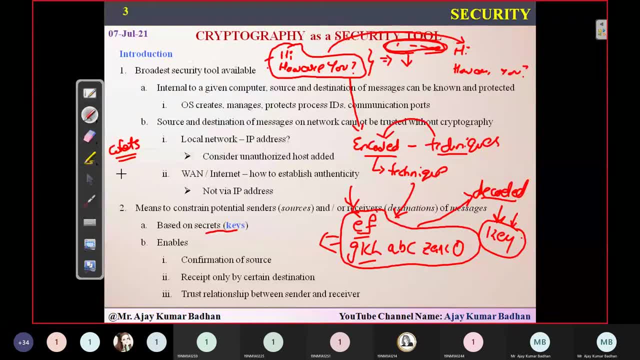 please type this: credibilityение c admire my message. inside the heli of you need background caionise. entering with respect to your friend. you will say that the security code has been changed with your friend's number. you did you see. there will be a hologram. there will be a hologram. 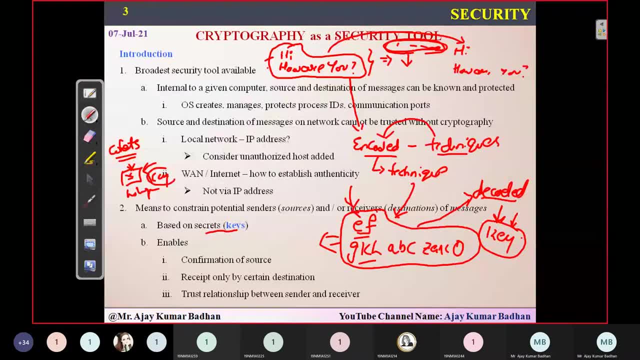 there and there you will be seeing that the security, if there is a security code, changes, this hologram will also change. this is the hologram, this is the key you can see. this is the only key which is present in between you and your friend: encrypt the data and send it up, and when it reaches your- so i mean your friend- she will be. 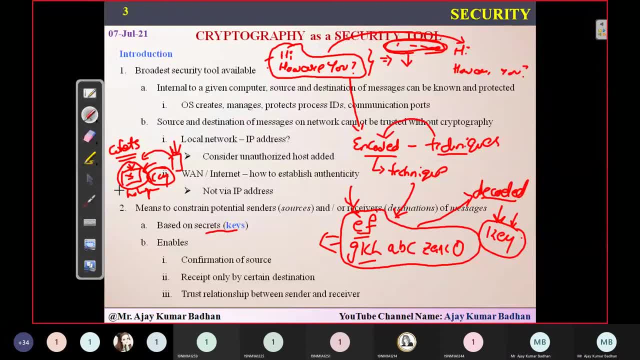 having the same key and using that key, she will be decrypting the data and finally she will get the actual message. now, in between, suppose a third person comes and he tries to get the information, he will be definitely getting this particular information, hacked information. so this encoded. 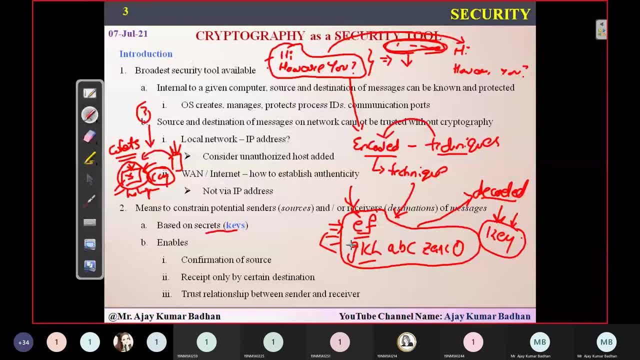 information, he will not be able to perform the operations on that why? because he don't know, he is not the one which is having the key. but in case, if he has that particular key then he can try to decode it. but he will not be having it because whenever there is a connection formed between two, 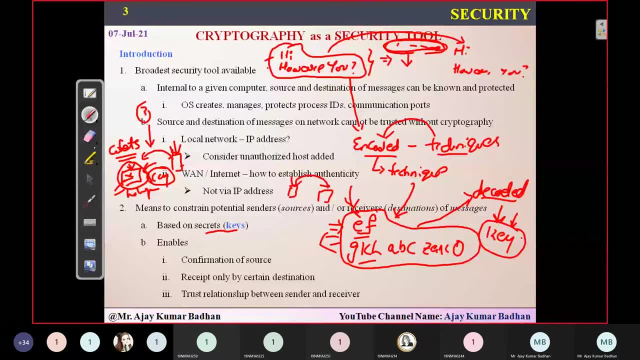 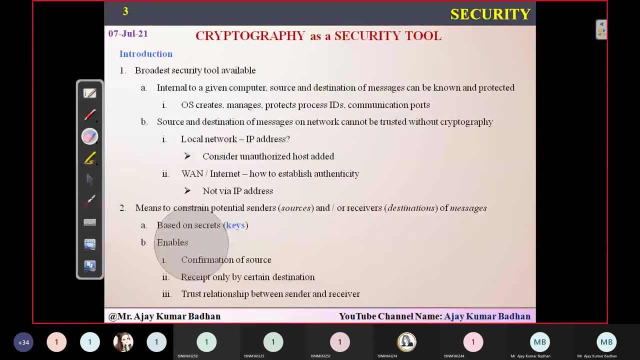 different source and destination. they both will be having those particular keys. okay, remember that. i hope you people are getting this. so the best example is a whatsapp group. you people might have seen. if not, you people can see. you can open one of your account. uh, number your friend's number. 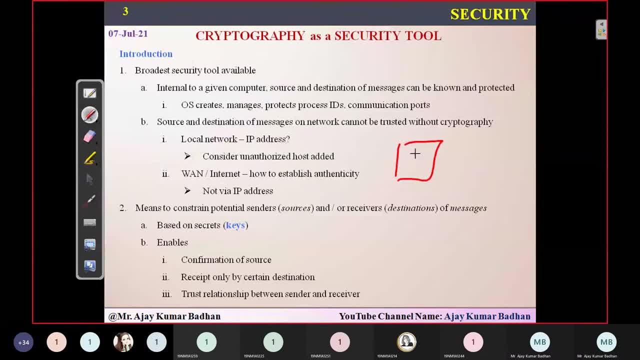 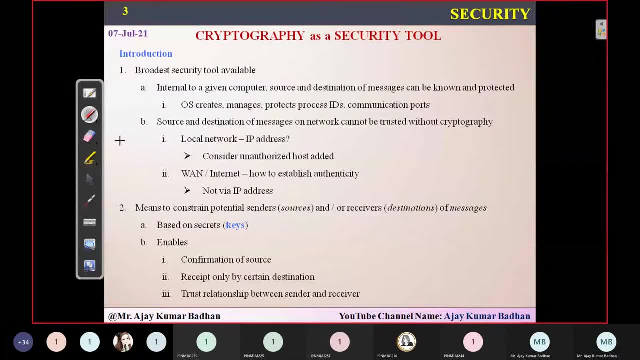 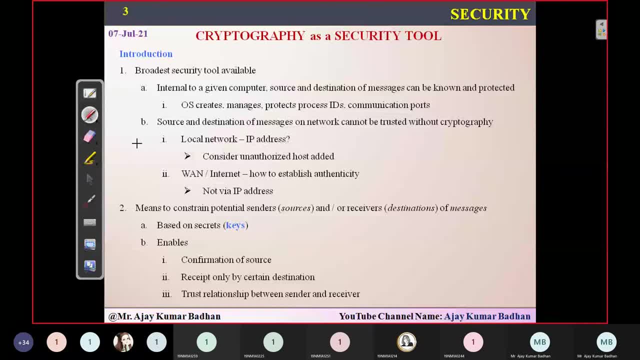 to a particular group. so whoever is present within that group, they will be having the particular key. so, okay, we are not using it by default, we are. that is present in the application, the. the application is designed in such a way that will consist of it and using that we will be able. 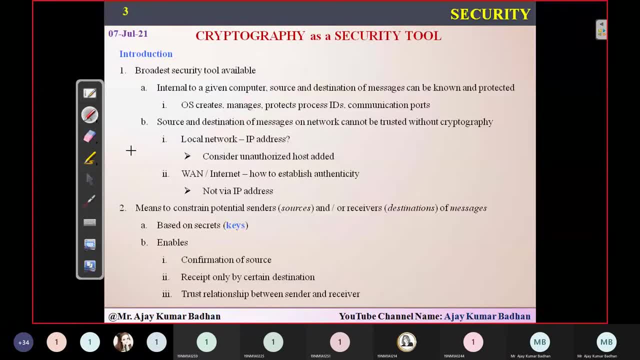 to see the different, different messages, whatever has been posed in that particular thing. so the only thing, what do people have to keep in mind here, is something called as keys. so key plays a very vital role. using this particular key only we people will be performing encoding of. 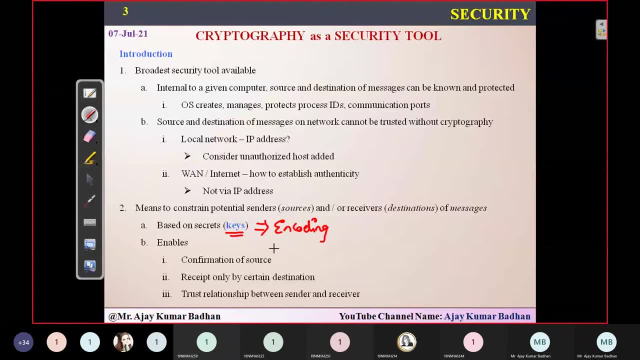 the data. whatever the data we want to transmit, we can encode it using this particular key. same way, using these keys only, we will be performing decoding of data. both will be done. so encoding will be done in the source from where exactly that message has to be transmitted. 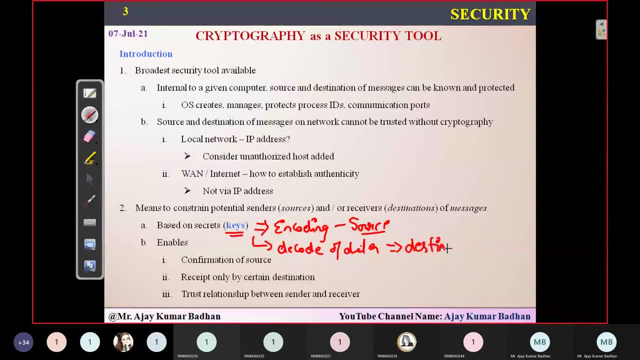 and decoding will be done at the destination. whoever you have intent intended to send that particular message, that is what you people have to keep in mind. so here, using this keys, what happens here? it actually enables three different things: confirmation of a source, so this key will confirm. 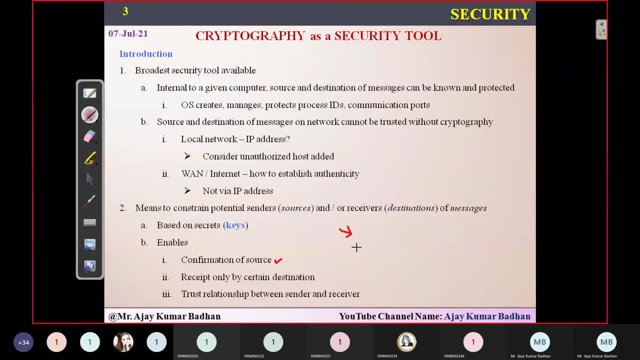 so whenever you people get a message from the outsider, so suppose your friend, so this will be confirming this key will come from. okay, this is from a normal customer. if not, it will immediately, uh, give you a alert that this particular person- for example, you don't have a account phone number- 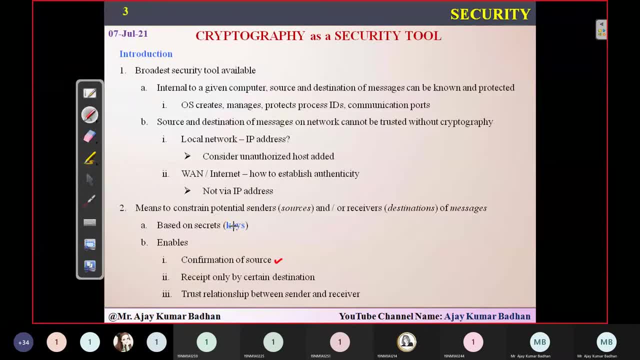 that is a present in your account. you don't have a phone number that is present in your account- your mobile phone- and suddenly you got a message from x person. it will simply say that this person is not available in your mobile. so do you want to save it or you want to delete it? that confirms. 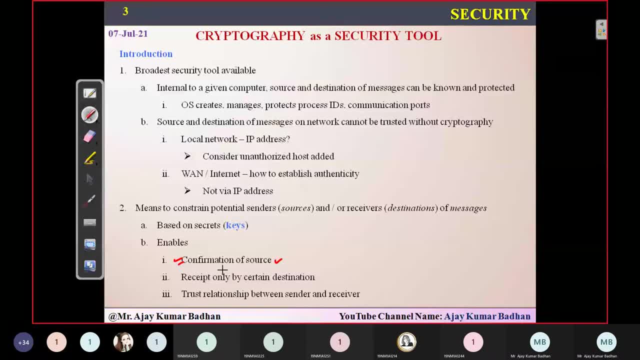 that particular source. if you don't know that person, what you will do? simply will ask to either delete it or block it automatically. this application will be blocking it up, but in case, if you feel like, okay, you know that person, then what you can do, you can store it as soon as. 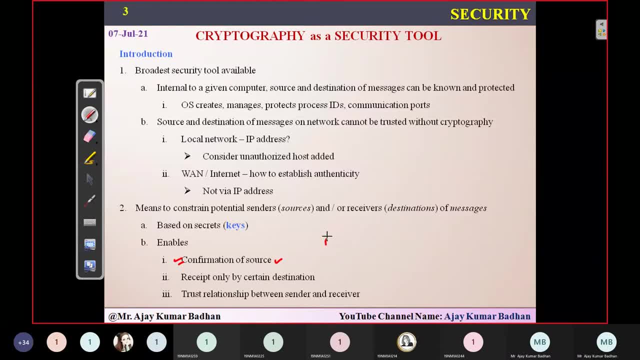 you are storing that phone number within your system, automatically a key will be generated between your app and between the person who has sent that. in between them there will be a keynote. this key will be shared between by source and destination. so next time, if you are transmitting, 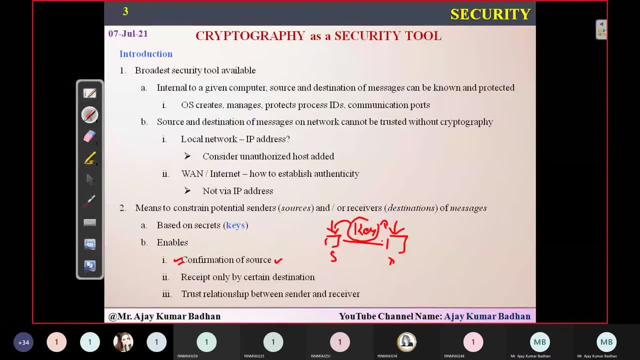 a message, or this person is transmitting a message. this key will be used for performing encryption operation. okay, and the next thing, what is saying, is: received only by certain destination. as i told you, whoever is having the destination key- i mean the key they only- will be able to. 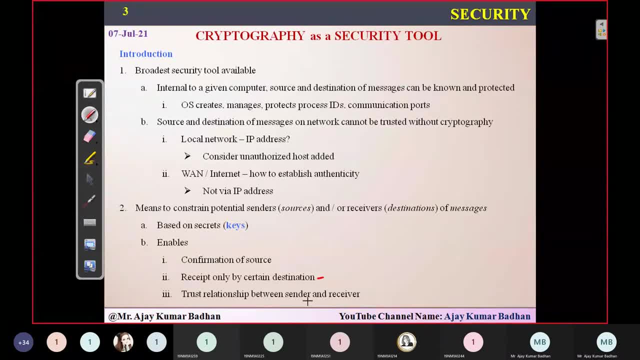 decode that particular code and they can use as a set. so trust relationship between centers. obviously, if you have that particular key, you people can sending an information from here to here and here to your source to destination or destination to source. that means you people are trusting each other. you may be sharing some critical information. 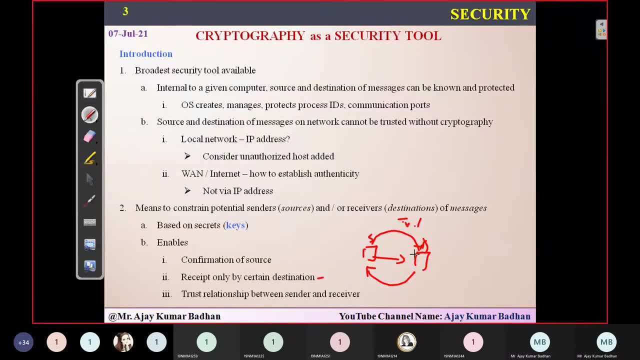 with your best friends or something like that. so what you're doing exactly, you're trusting it. that, okay. this so when you're transmitting that message, okay, you're trusting your friend. but you, the way you people are using, what kind of application that is? also you have to trust, for example, in: 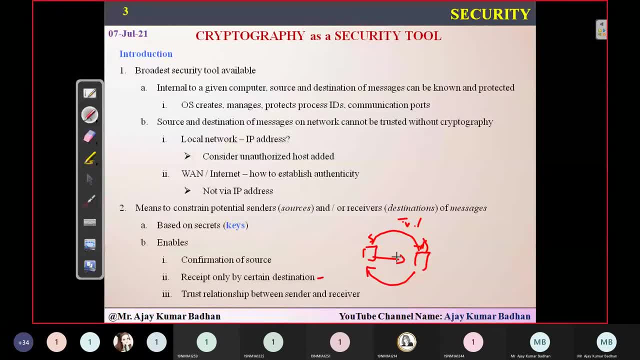 whatsapp. if people are transmitting the data. so it means what does that mean? you're trusting that, whatever the critical information i'm transmitting using this particular application, that will be secured. no one can access that particular data. that's why people are transmitting it. if someone can hack it or something like that, if the reputation is not good, then will you be using? 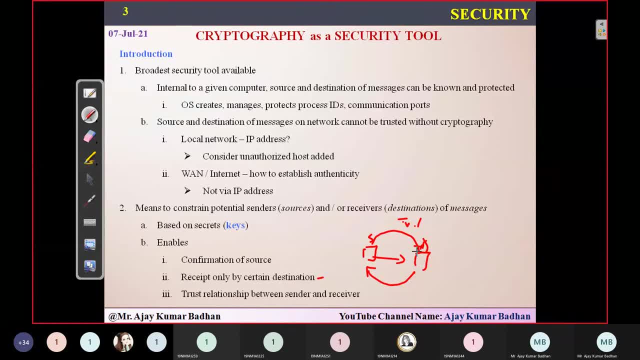 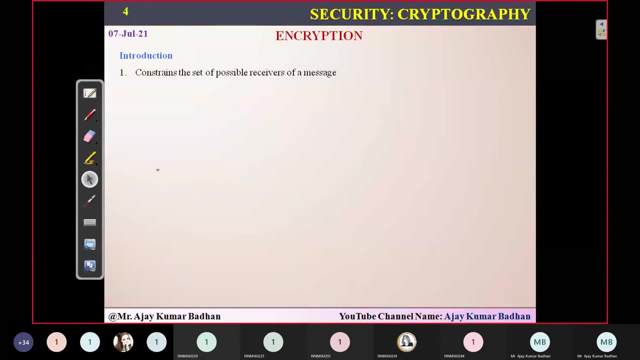 the same application for transmitting the data from that particular application. no right, so that is what he's talking about in this particular. so these are the three things that enables this particular key. so let's go ahead. so now comes the encryption. so what exactly we are going? so i'm telling you that we will be encoding the data. encoding the data. 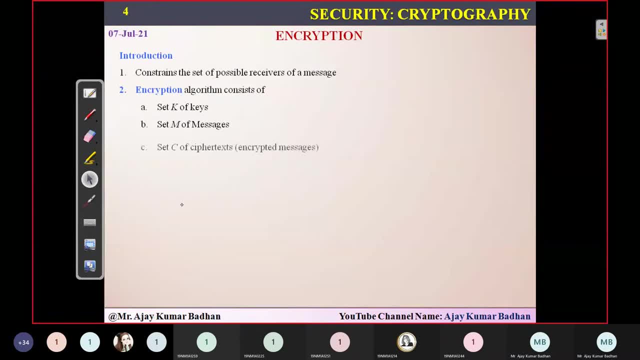 and all. what do you mean by encoding? here is nothing, but we call it as encryption. so we are going to discuss this encryption here and then we'll go for the other part. okay, so here, if you talk about encryption, why we are using this encryption- the best thing is we are using this to. 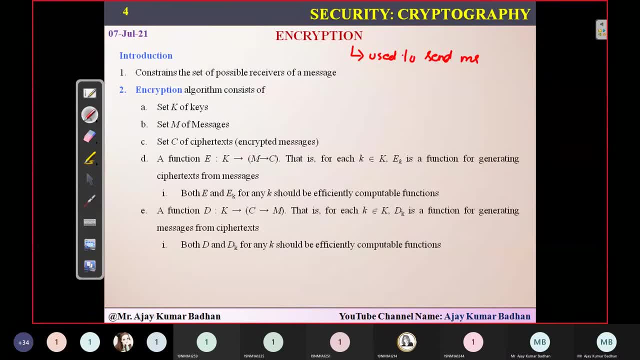 send the messages, like if people are transmitting messages using whatsapp- normal messages or your messages or whatever. so to transmit the message from a particular source to a particular destination, we use this particular technique called as encryption. what it will does is nothing, but it is the one which will be performing encoding. it is the one which will encode the. 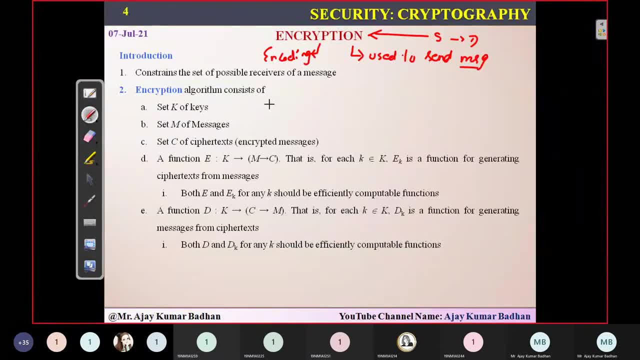 data, whichever we wanted to transmit it up. so every encryption technique will basically consist of these three points. you people have to remember this. it will actually consider these three components. what is the first component is a key. as i told you in the beginning, secret key. so it will. 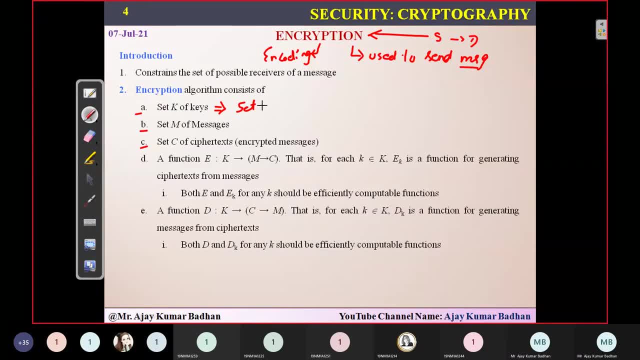 consist of set of keys. okay, so it will be consisting of set of secret keys here, and that i'm representing with the capital k set. remember it is a set set means there will be some multiple number of keys. then we have something called a set of messages. so these are nothing. set of messages. 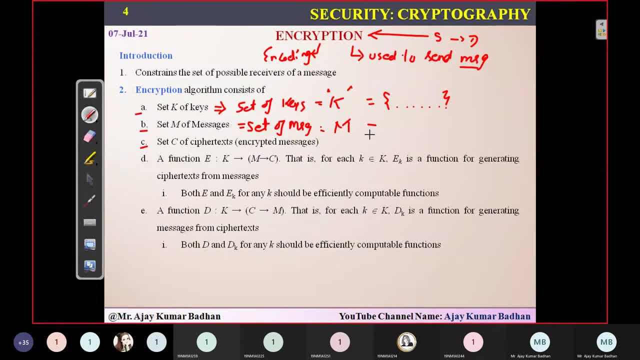 in the sense we are representing with capital m. so what name? the set of messages here are nothing but, like you people are transmitting hi, how are you? and after that you're in the same message. you're typing that, uh, be ready by 5 pm to go out something. this is a message you people are trying to send in a single stretch. so what? 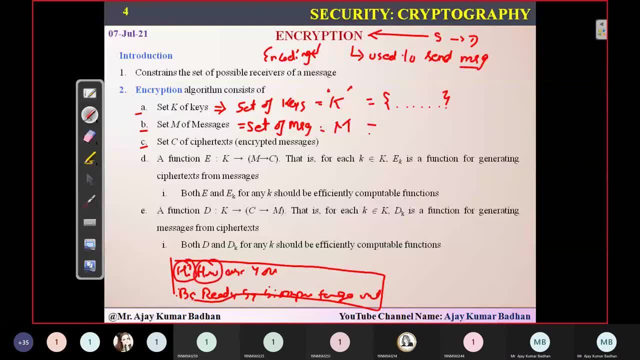 happens here. these are the set of messages. this high is one message. how is separate packet r is separate packet. use a separate packet this way. so what happens here, each one will be, will be considered as a set of messages here. so that will be represented within the curly braces, that is. 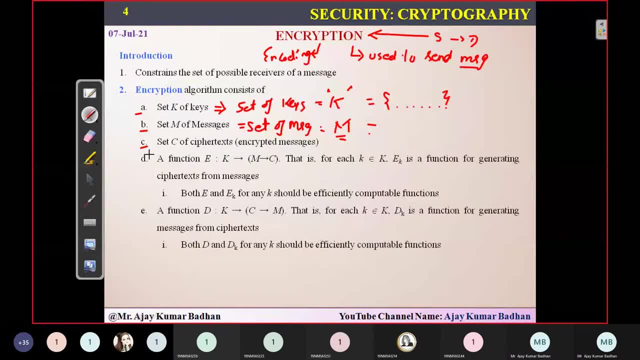 what he means to say here. and then we have something called c. c is a term we are using to represent cipher text. cipher text to i don't know how many of you heard this name. well, cipher text is nothing. but m is nothing. but it's a normal message. normal message, something like, as i told you, hi, hi. so this is a normal message. 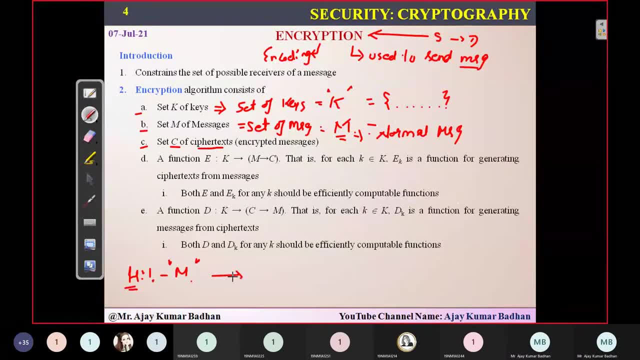 and once you people are using a key to encode this particular message, you will be getting a cipher text. okay, text like you may be getting so high will be converted into something called as ez. and oh, let us suppose zero, e, z, zero. what do you mean by ez? zero is nothing, but this is high exclamation. 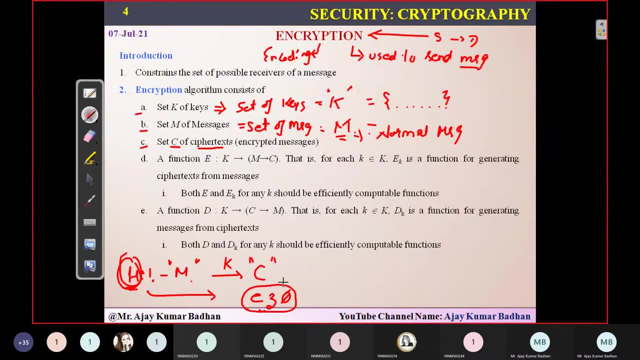 mark is represented like this. so this you people will not understand why, because this is an encrypted text. that's what we call it as a c cipher text. okay, whenever you people are converting a normal text message into an encoded format, that message is what we are calling it as cipher text. 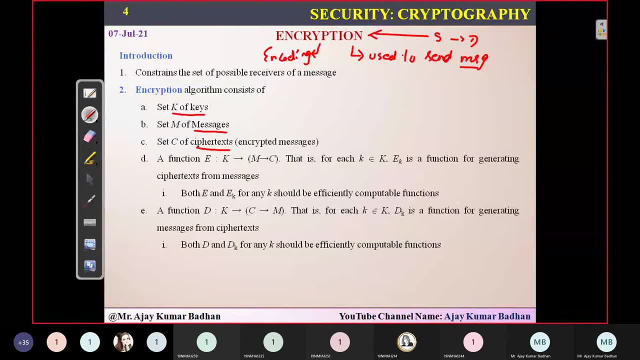 normal messages are represented as message and these are the keys which are used in order to convert a normal message into a cipher text. so in order to do that, definitely we need some function here. so the function, what we are going to use here, is something like this: we have to use two. 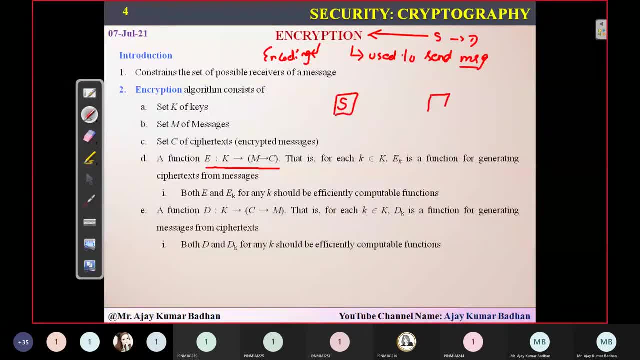 different functions: one in the source end, another at the destination end. source end, we'll be using encryption function and the destination end we are using something called as a decryption function. so we are going to use a decryption function and we are going to use a decryption function. so what is the encryption function we are going to use here is nothing. but whatever the 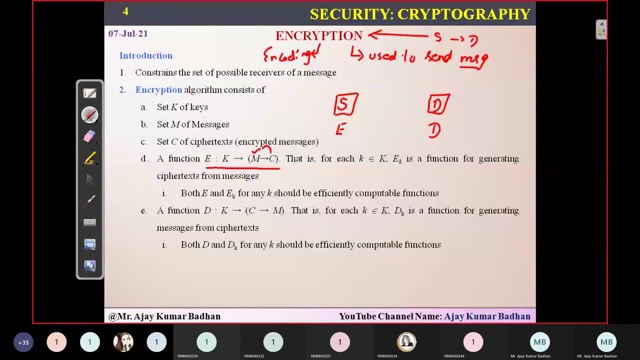 set of messages we are having here. we will be converting that into a cipher text messages set of cipher text messages, and how we can do that using a set of keys that are present into this particular value. okay, so in this, as i'm telling, this is a set of keys right k, capital. 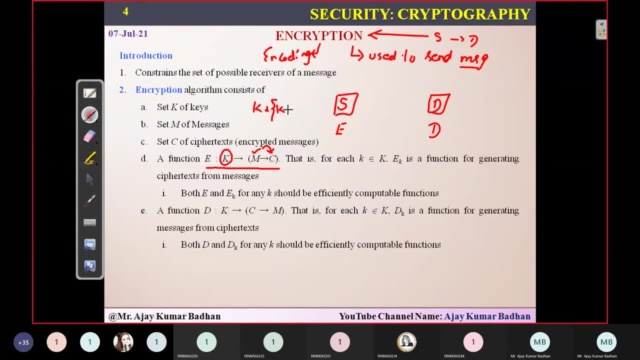 k represents set of keys, so that keys are represented as small k, k 1, k, 2, k, 3, so on, what are these small k 1, k, 2, k, 3. these are the keys, set of keys, what we have. so i am representing. 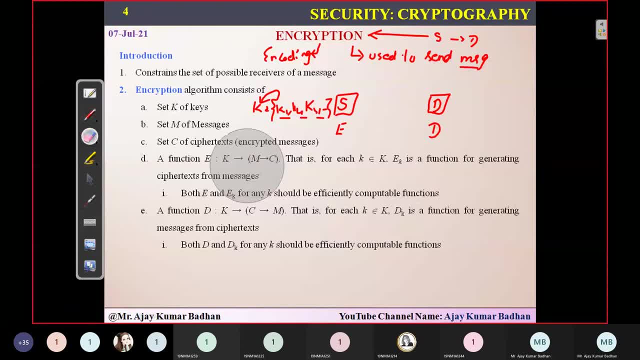 with capital. so, see here, that is what is representing here. so this is the function we use for encryption. so, using a particular key from one of the key, from this particular set of keys, we will take one of the message from this particular set of messages and then we'll. 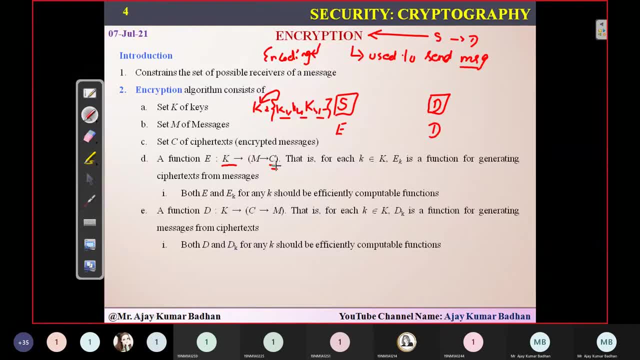 directly convert into one of the cipher text. we'll be directly converting into a cipher text now. here small k is nothing but belongs to capital k. now i think you people might have understood what is small k here. this is: a small k is nothing but one of the key. 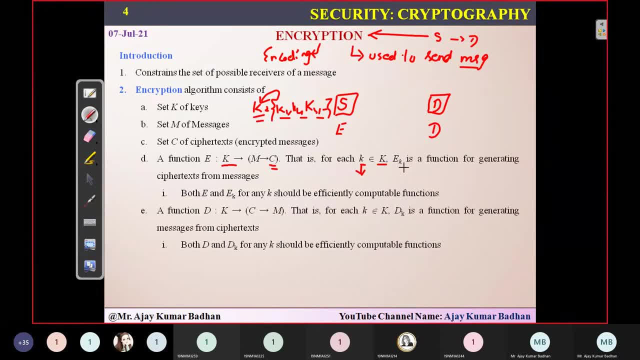 from this particular set and ek is nothing. but this is a function. now, this whole function, whatever i'm showing here, this he is representing as ek. what is this small k? so, using this key, we have used this particular function and we got a new cipher text. okay, so this is what he's saying. 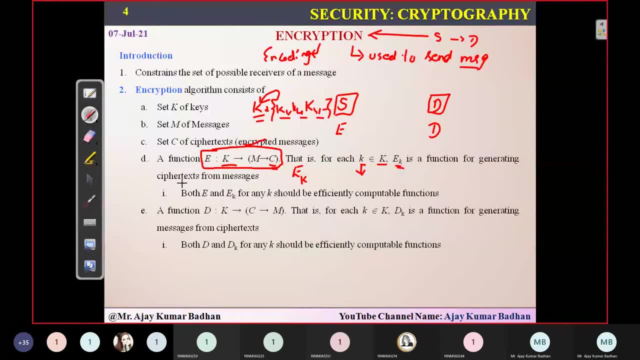 here. this is a function. ek is nothing, but it is a function for generating cipher text. for what? for the normal message, whatever you people have typed in your system. okay, i hope you people are getting it. so here both. this key is a normal function, encryption function. ek means that encryption function you are implementing. 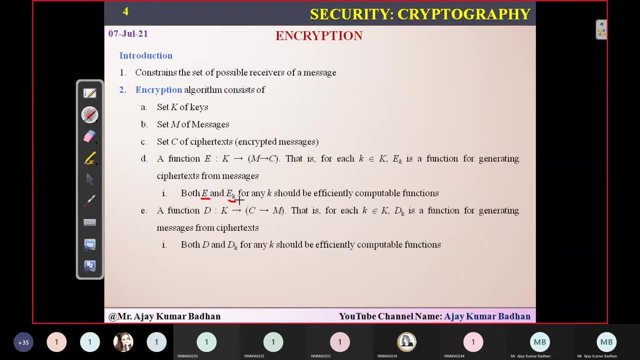 using one of the key from the set of keys, what we are having here, so this is useful. this is sufficiently computable function so we can easily compute this. that is what is saying here now. next is decryption. decryption process is same, only thing these two variables will be changing here. 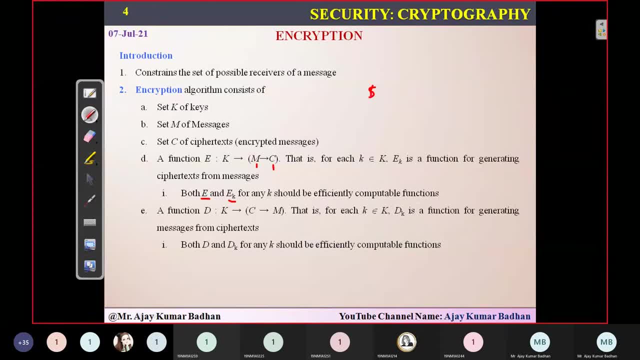 decryption means what you have to do. you will be so here. when the source person is sending the data, he will be encrypting it and he will be sending it. so when you are encrypting a data, what does that means? it becomes a cipher text. now that cipher text will be reaching this particular 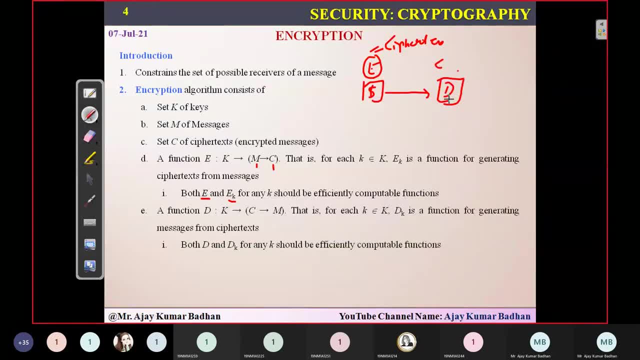 destination that cipher text is, but this cipher text he cannot read. so definitely this cipher text, using the same key which you people have used here to encrypt it. using the same key, they have to convert the cipher text into a normal text, that is, m, and then the destination will be able to read this particular message. 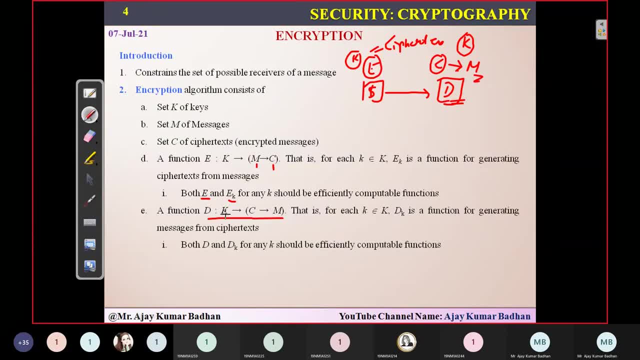 so this is the code for that. this is a function. we are using k, so using one of the key from a set of k- i mean set of keys, what we have, whatever the cipher- i mean cipher text- we have received at the destination, will be converted into a normal message. okay, so at the source end we'll be. 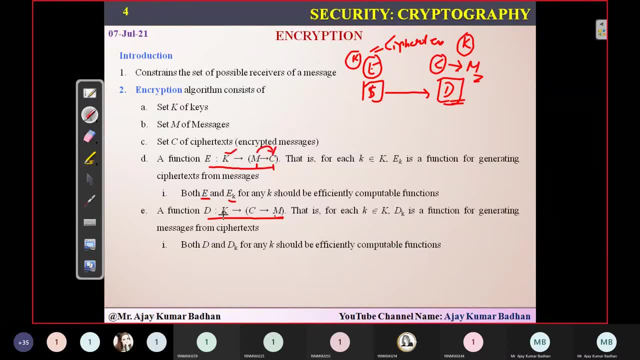 converting a normal message into a cipher text using this particular key and whereas, coming to destination, we'll be converting a cipher text into a normal message. and then the destination, we'll be converting a cipher text into a message using a normal- i mean using that particular key. 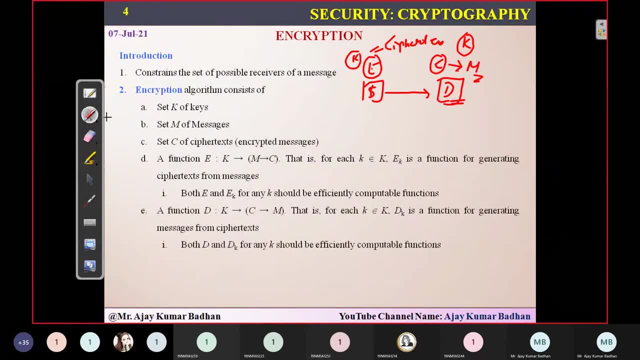 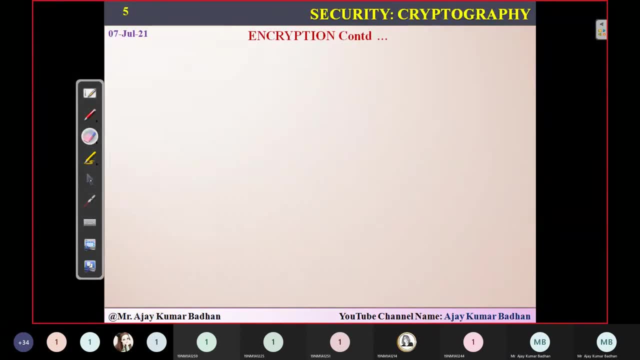 same process, remaining both the same, what he is talking about here. okay, so this is that normal technique, what we exactly use in order to implement it. so here, in this case, when we are implementing this, uh, definitely, we have a functions and all right. so there are certain properties that 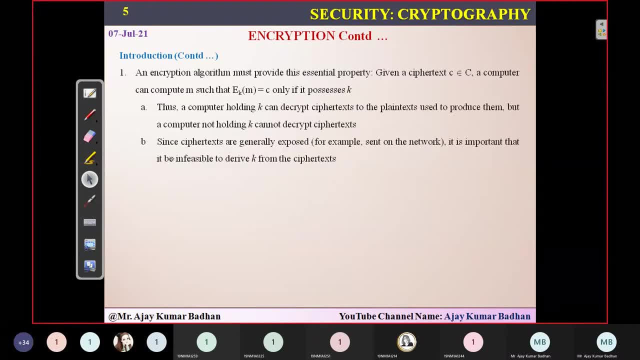 we need to consider when we are implementing it. yeah, oh, sorry. so there are some properties that we need to take care when we are implementing this. uh, let us suppose that your system, your computer, is computing a message, means it is trying to convert this message. you are having some message something like: hi, how are you? whatever it is so on. 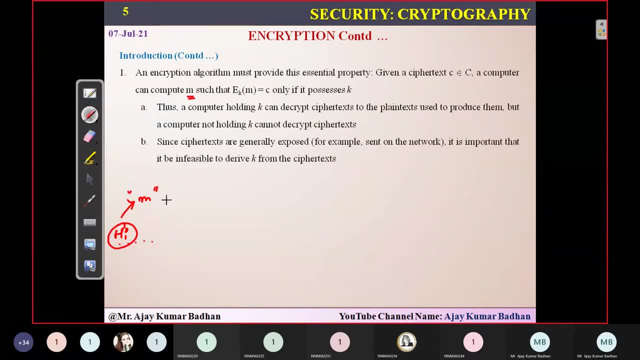 this message i am representing with small m. now this message i want to convert into a cipher text so that i can transmit that to my destination friend, whoever it is. so here the concept here it is ek of small m, so means i am going to apply a function, encryption function. we know that. what is? 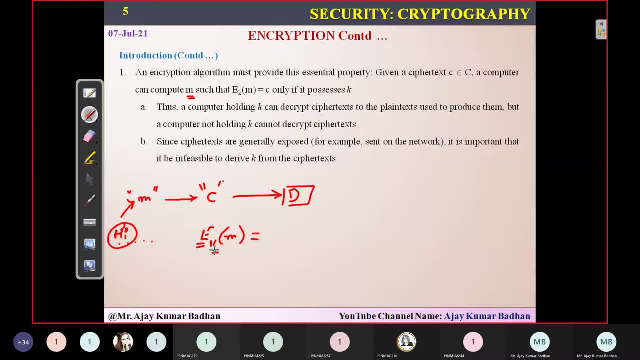 an encryption function using one of the key from a set of keys, what we have, and i will be using that key to encrypt this particular message, this is a message, actual message, hi, and this message then, finally, will be converted into a cipher text, and then that particular text will be transmitted. 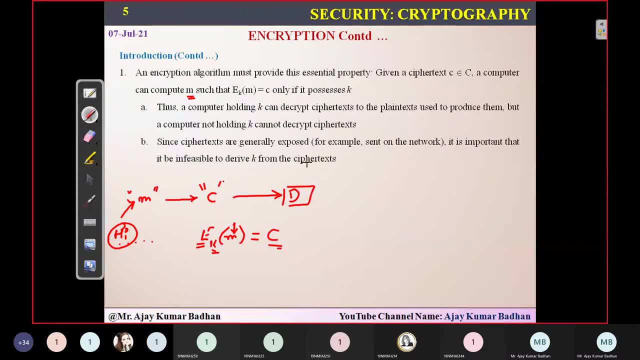 this particular cipher text will be transmitted to the destination. now, here, the system, your friend, whoever it is, he will be having the same key. this small k will be. whatever the key i am representing here, this key will be present with this particular destination and this message will. 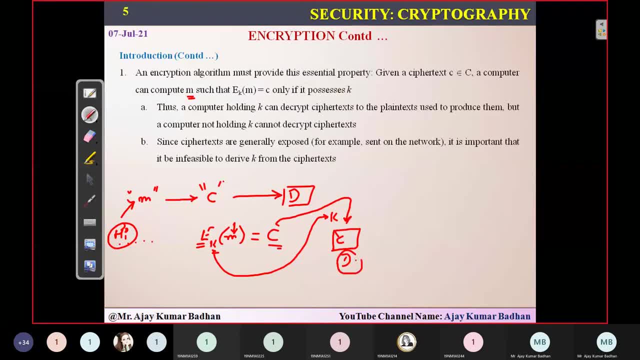 be reaching to the destination here now, what this particular destination will do. he will be applying this particular key onto this particular cipher text and then, finally, he will be able to get the actual message, whatever is there, and then he will be able to read the information, and this is a 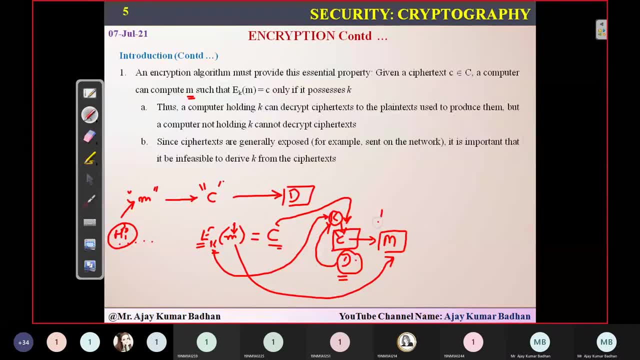 vice versa. format means after reading it. definitely, if you say hi, they will also respond hi, how are you? so? this will be transmitted from here. so when he is transmitting here from destination, he will be encrypting using the same key. now, this time, the destination will be encrypting this message and 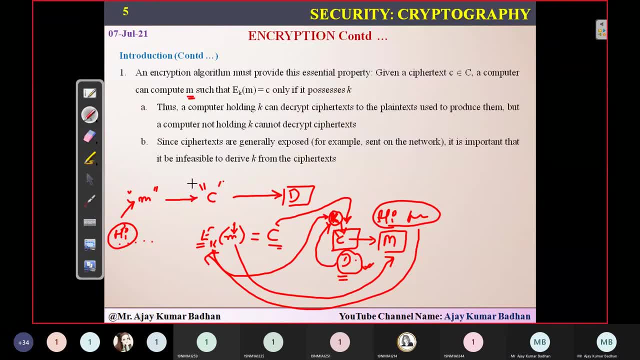 he will be transmitting it now, since the- uh, what we call the you people means you being the source node here, you're also having the key, so obviously you people will be able to decrypt that particular code and you will get the information, whatever it is. hi, how are you then? you will be replying it. 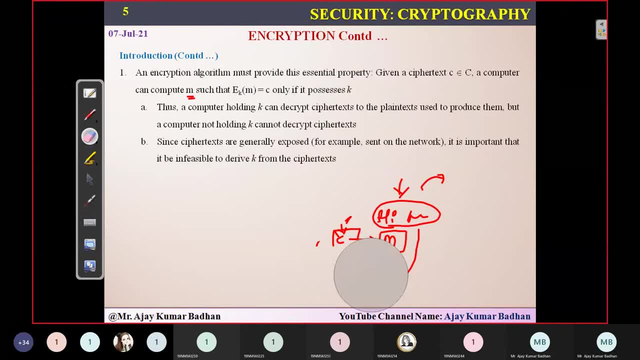 so every message you people are transmitting over the network is nothing. but if people are encoding and transmitting, and how we are doing it with the help of our technique, we have something called as encryption. okay, so there are some techniques, as i told you, so one among them. 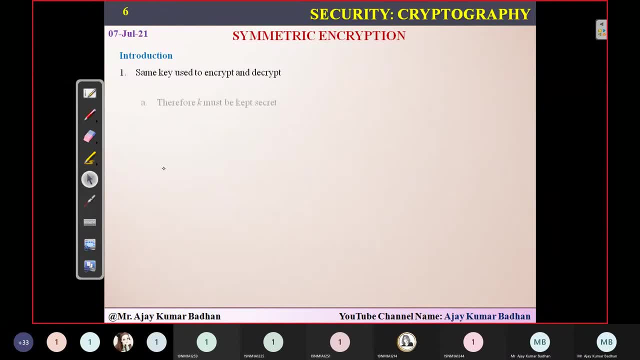 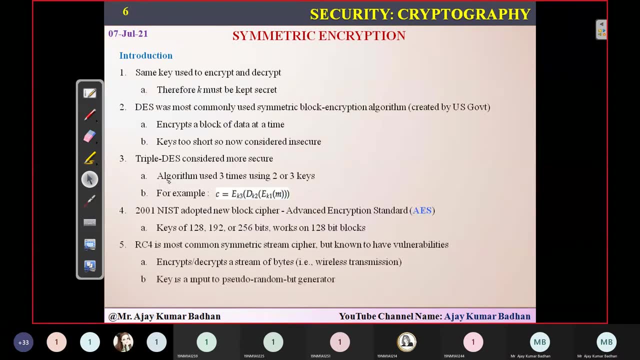 is symmetric encryption. they're actually okay, let me show it up and then i'll explain it. okay. so actually, you know what? uh, this encryption is basically classified into two types here. one is what we call it as symmetric encryption- symmetry as encryption- and another one is what? 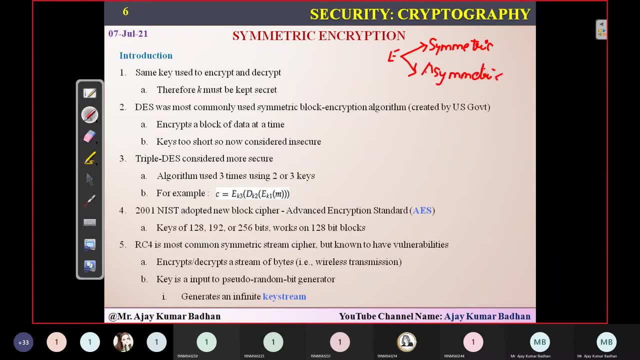 we call it as asymmetric, asymmetric encryption. this is what we call it as a symmetric encryption and this is what we call it as asymmetric. now, the one which we are going to discuss right now here is something called symmetric encryption. okay, the first one. so what exactly it exactly? 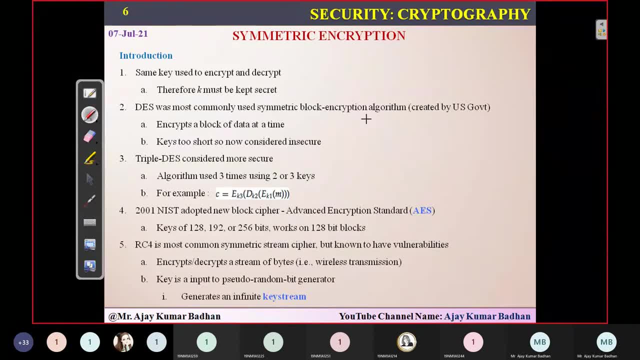 about this particular symmetric encryption is here. the same key will be used for encryption and decryption. that is nothing but what i have just previously explained it. so here you are. the source node. there is a destination node. he will be transmitting the message, so he will be having 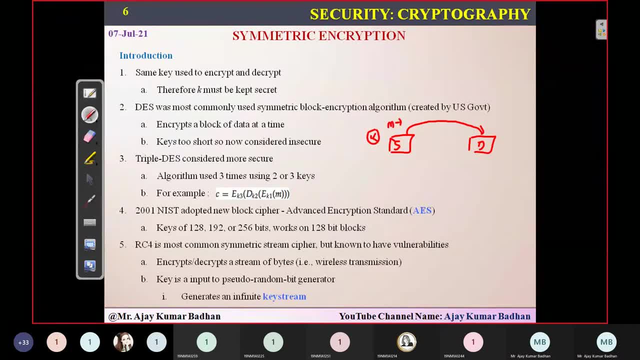 some key k. using that key, whatever the message is there, he will convert into ciphertext and will transmit it. this ciphertext will be received by this particular destination. now he will also possess that particular key. so, using this key applying on the ciphertext, he will get the actual message: what is, what did? i also told you that this is a vice versa. so after getting the message, 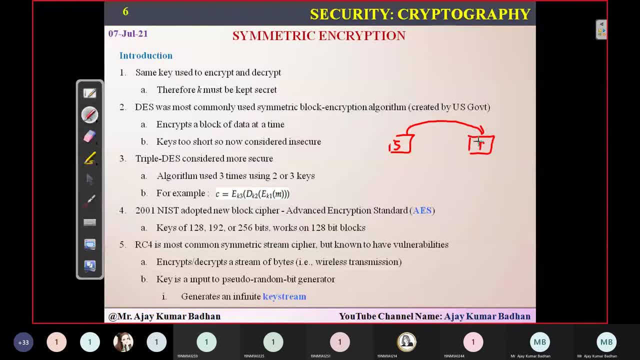 what. what will exactly happen here is: the destination will be giving a reply to this. so when he is giving a reply, he, he is going to send a message. now this message will be converted into ciphertext using a key and then it will be transmitted. now this source node will be getting a. 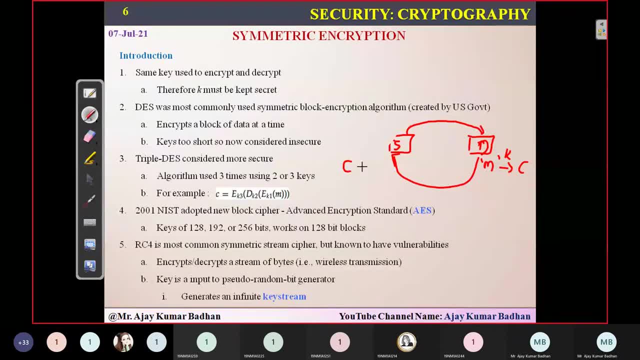 encrypted. encrypted text here, that is ciphertext. now this ciphertext will be converted into a normal message using the same key which he is having, so both are sharing this particular key. since i am telling that this is a single key which is shared by both of you means the source node and the destination node. both of them are sharing the same key here. 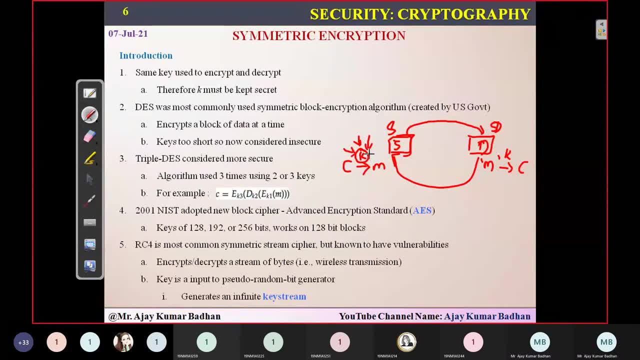 so definitely you can understand the importance that this particular key has to be protected. this key should not be known to the third person. if the third person knows about this particular key, automatically he is going to what is going to do? he is going to automatically decrypt that message. 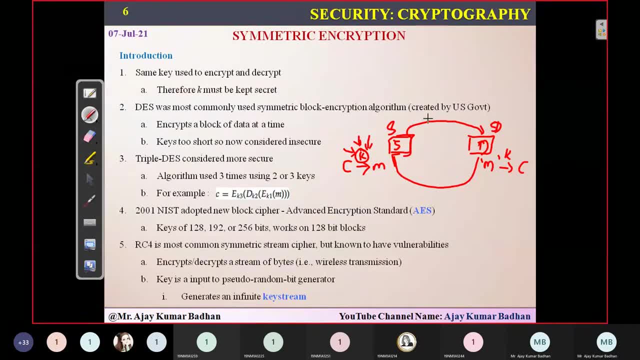 and he will be getting the information, whatever people are transmitting it, and there is a possibility he may try to modify or he may try to do some kind of infringement with respect to the data, whatever you people are transmitting, so that people have to keep in mind when we are performing it. now moving ahead. so here, apart from 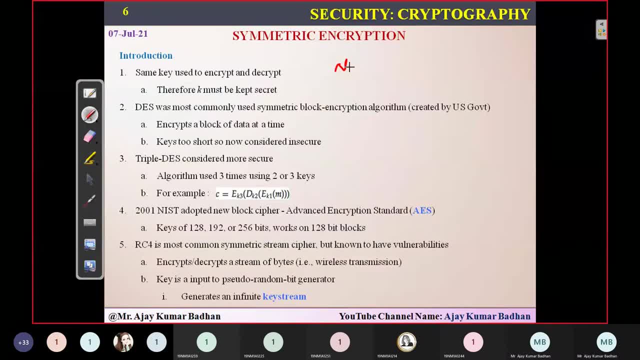 this uh earlier. we, as i told you that nist is the organization which actually developed this, so they are the one we. they use it, this particular uh, what we call encryption technique. so the most common technique, what they used to have is something called as des algorithm. they use des. 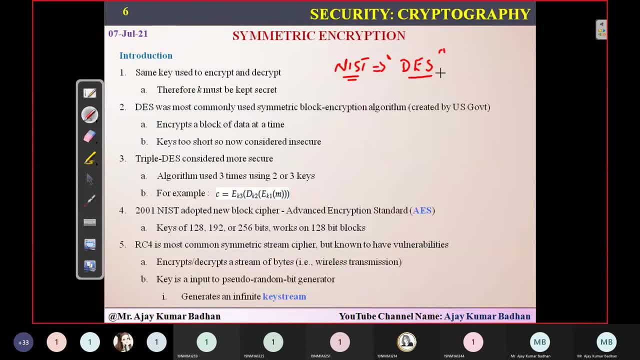 data encryption standard. this is a one which is used in order to convert a normal message into a cipher text message, and this has been used by home nist national institute of standard and technology. but, as you know, the technology has progressed. the hackers are able to detect whatever the 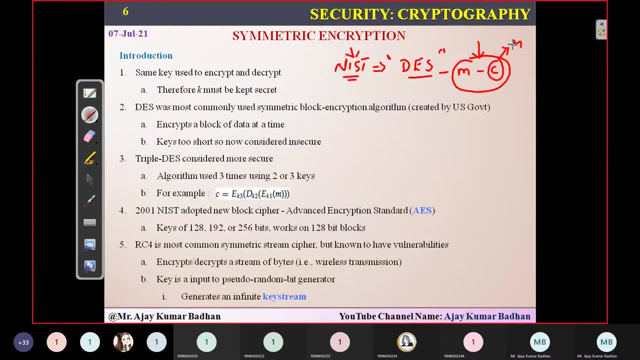 message ciphertext. is there this ciphertext message? whatever the actual message here, they are able to decode it okay, without having a key. also, you know, as a technology getting advanced, automatically they'll have some loopholes and based on that, they used to identify it. so what this particular nist did is, rather than removing this ds algorithm, since it is no of no use in the 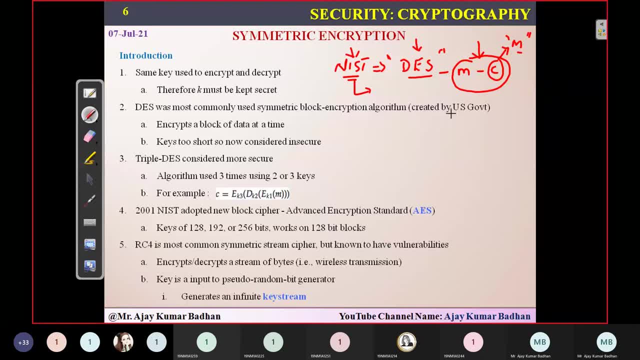 further. they just try to modify this particular ds and they have implemented. how did they modify? here is nothing but the same algorithm. they applied three times on a particular message. first what they did- ds algorithm- they applied only one time. so whatever the message they want to send, 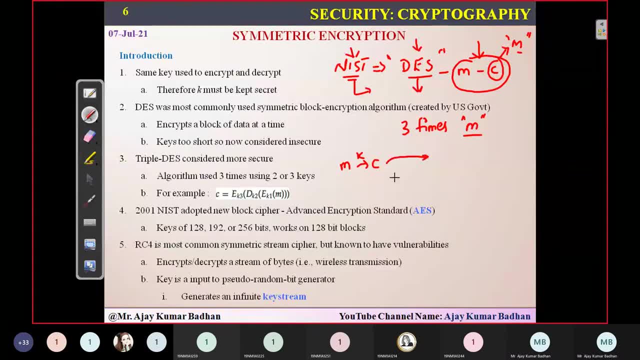 they applied using a key one time and they convert into cipher and that is transmitted. but now ds, after certain time they started implementing. three times means first there is a normal message: they applied a key here, they got a ciphertext. now, on this ciphertext again, they applied the same key, they got cipher. one means much more advanced. 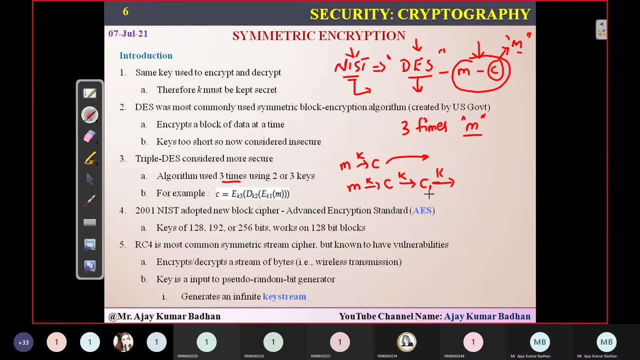 and again. on that they applied, they used the same key and again they encrypted this message. now they finally got c2. now this c2 will be transmitted to the destination. so in the destination also same process. when he receives c2, he will be applying the key and he 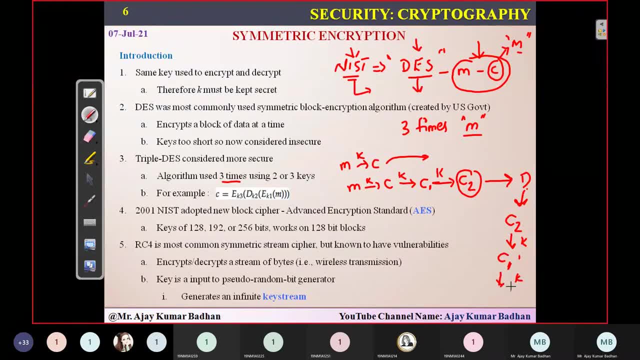 will get c1 again. on that particular c1 he will apply the key and then again he will be getting that actual output. okay, so whatever the actual message is that he is going to get, so three times, they are going to apply it so that they can get that particular thing operation. now here how they: 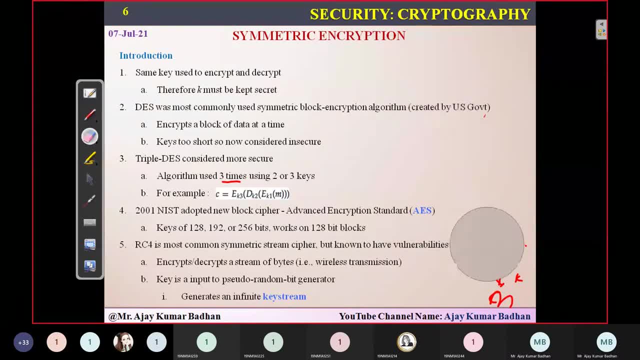 exactly applied. the question is how they exactly applied this particular thing. well, they, they have some techniques here. so the technique, what they exactly have here, is that they use- suppose you want to send a message, the size of the message. they usually used to take something called a 64 bit. 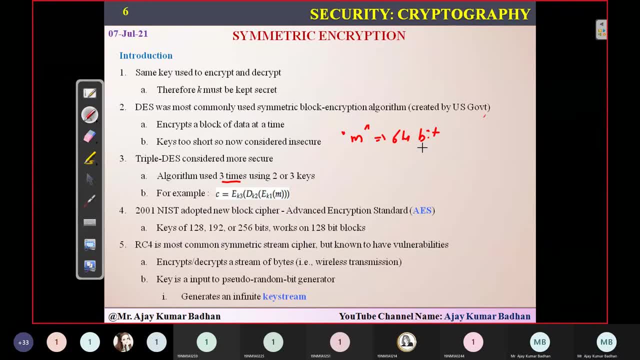 remember this. so first time when they applied only single ds algorithm- and they used to apply it, they used to take 64-bit message, whatever the message size. suppose if your message size is 128 bits, they will initially take first 64 bits and they will encrypt it. so definitely we have to. 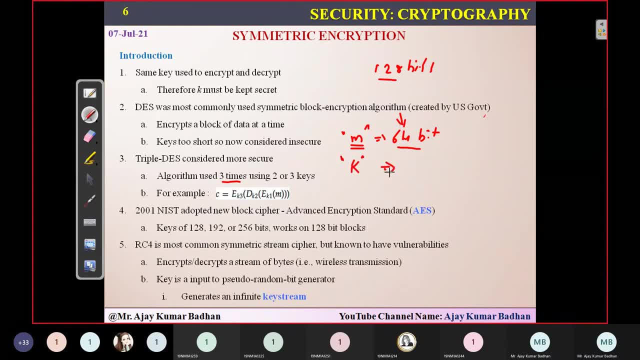 encrypt. it means we need a key. so the key is nothing. but that is also nothing, but it's a bits. so how many bits they used to bit key is 56 bit key. they used to have a 56 bit key. using this key, they used to encrypt this particular message. as i told you, m you're applying a key, you're. 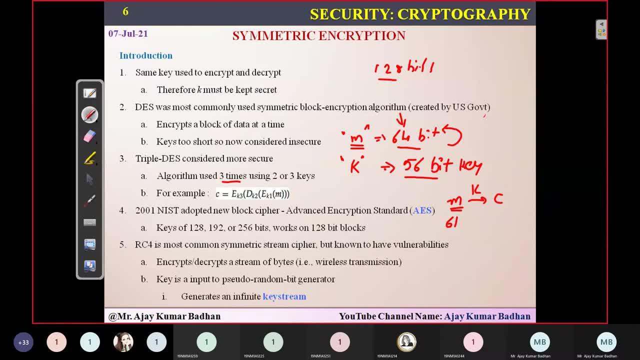 getting a ciphertext. so what is the size of this particular message? whichever we can encrypt is 64 bit, and what is the size of the key? what we can use here is 56 bit. so using a 56 bit, we are able to encrypt a 64 bit message and we'll be converting into a ciphertext. this is the first one we used. 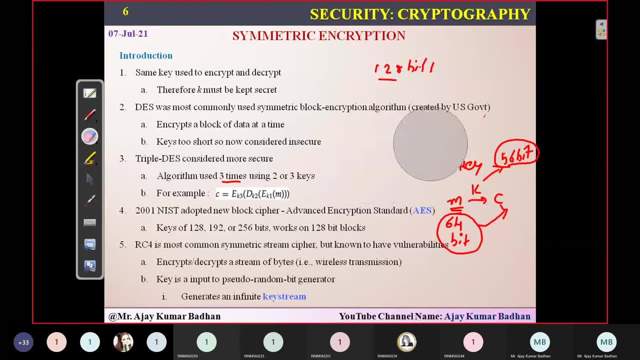 and, okay, you may be getting sir. okay, using a key, they are performing this ciphertext, how they are doing it? okay, so this is a very simple thing you people will be learning. uh, you people might be learning in your know- analytics, i mean for placements your people will be learning about. 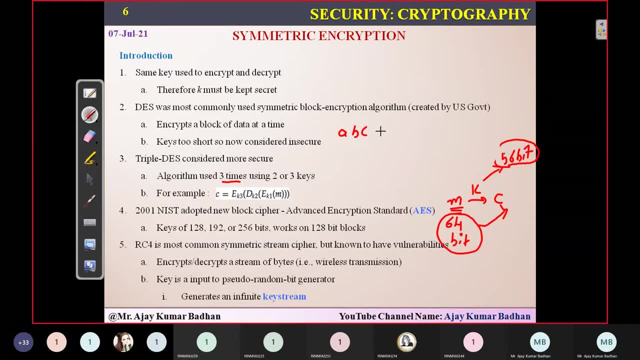 something like: you know, if a, b c, uh, there will be some mathematics like a b c, i am represent. okay, sorry, not a b c. yeah, yeah, okay, fine, if a b, c is represented as d, e, f, so how x, y, z will be represented? so can you understand this? how exactly people are doing so you have to find. so a. 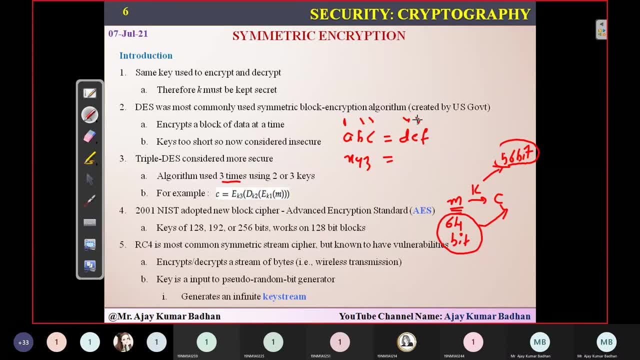 a is one, so d one, two, three, four, five, six means one plus three is equal to how much four, and this is two, right. so two plus three is how much five and c is having a value. three, three plus three is how much value six means. if i give x, y, z, you should know the value of x. so suppose z is 26, 25 and this is your 26, 24, 24. 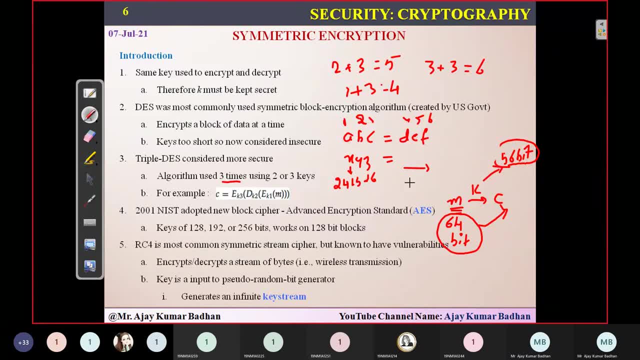 then what will be the output now? can you under can, can you get that, or uh, what we call the actual output now? so 24 plus 3.. so 24 plus 3 means how much you're going to get. 27. that is nothing but a. 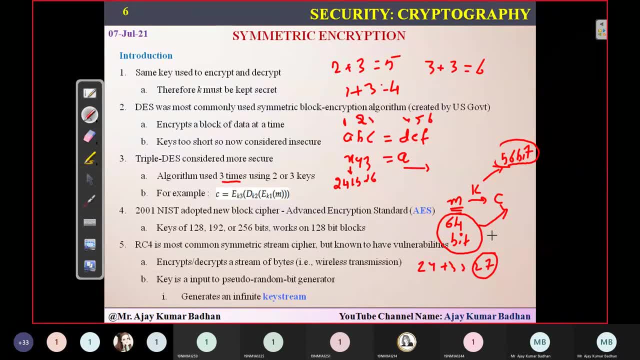 in alphabets we have 22, 26, so after 26, 27 means that is the first letter, a, a you're getting, so y, 25, so 25 plus 3, 28, 28 in the sense the second element. so we have in uh alphabets 26 alphabet. 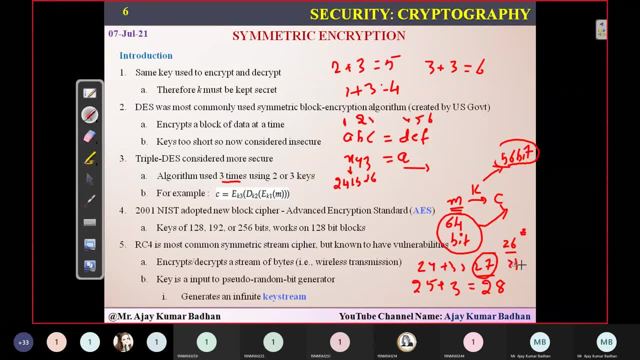 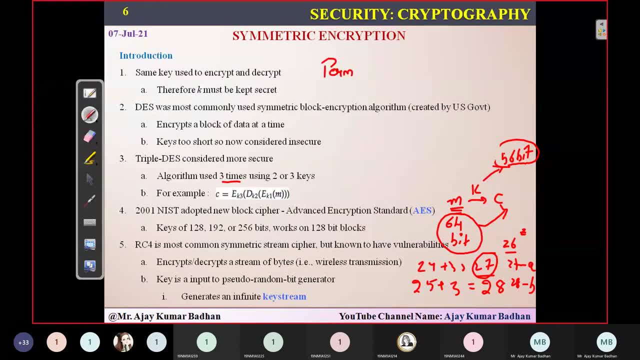 to do so here. what they used to do so here. what they used is nothing but simple mathematics is nothing but simple mathematics is nothing but simple mathematics. that is nothing, but we call it as that is nothing. but we call it as. that is nothing, but we call it as permutation. 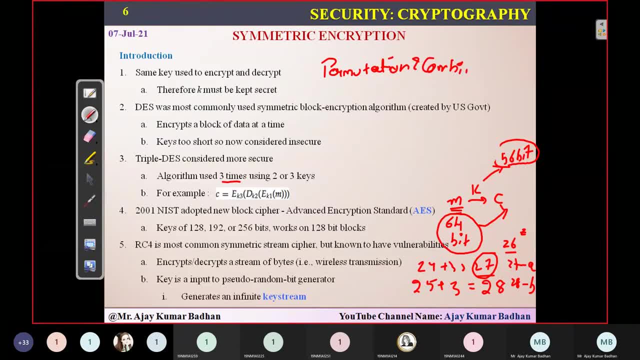 permutation, permutation and combinations and combinations and combinations. this people might have learned in your, this people might have learned in your. this people might have learned in your school time, in your college. i mean in school time in your college. i mean in school time in your college, i mean in either in the intermediate colleges or 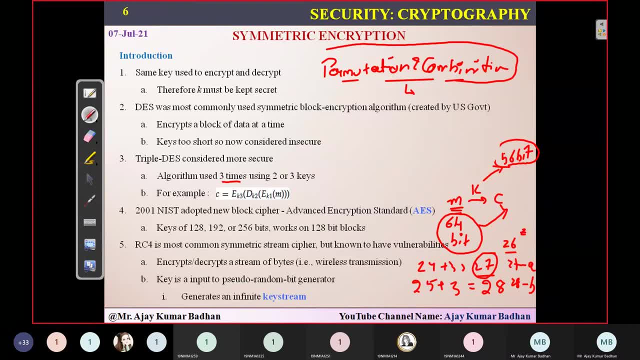 either in the intermediate colleges, or either in the intermediate colleges or during their 10th class- normal during their 10th class, normal during their 10th class, normal permutation comp. so using this permutation comp, so using this permutation comp, so using this combination, they actually generate, using 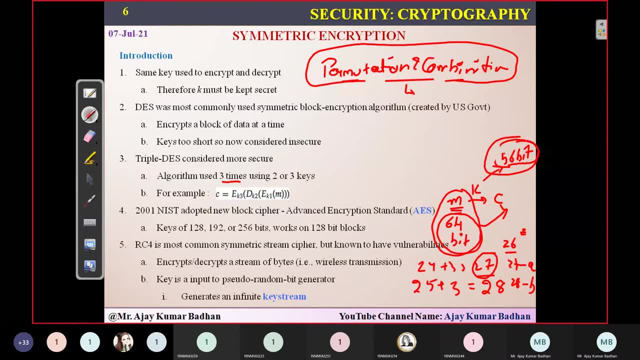 combination they actually generate using a 56 bit. uh, they used to convert into a cipher text or 64-bit message. this is the way they exactly used to do it. i hope you people are getting it. so how exactly they used to do it. okay, so i will show you one algorithm and then i'll explain it. that then you will understand much. 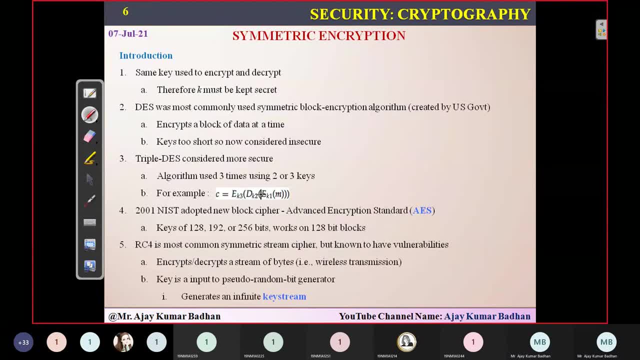 more easier, but that will be with respect to asymmetric, not symmetric now. here, uh, when they applied for three times, like, for example, as i told you that they used to apply three times here, this is the function they used. so to get a cipher text, they used to use encryption function where 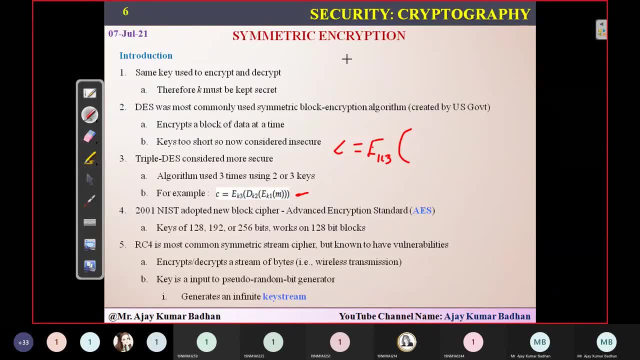 they applied three different keys. so what are the three different keys? so what is the three times they have performed that means? what does that mean? is two times they used to perform encryption, two times they used to perform encryption and one time they used to perform decryption. okay, so triple. this is what we call it as triple ds. 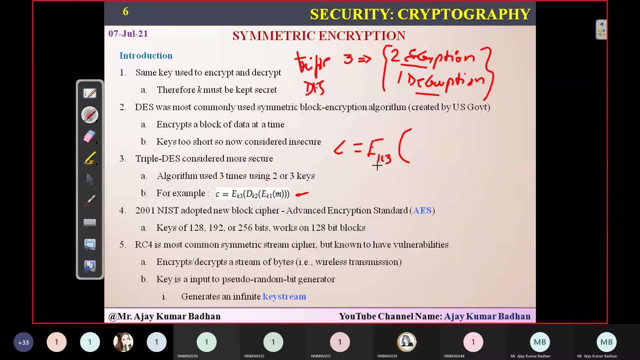 triple ds is nothing, but two times they used to apply encryption and one time they used to apply decryption, and that is what you're doing. so first time i'm encrypting it using a key number three, then using a key number two, i will decrypt it and then using again- uh, next key number one, i'll again encrypt. so this: 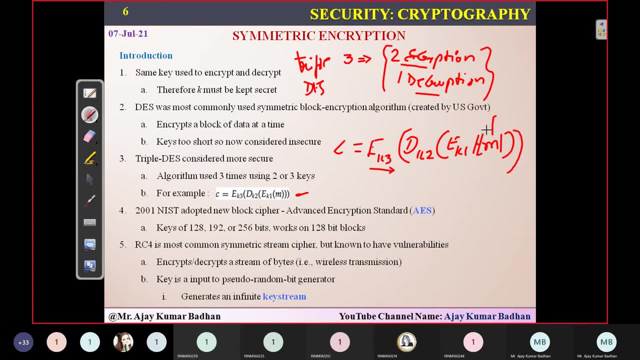 is the formula, what we exactly have. so what we are doing is: this is the actual message. so this message, i'm going to encrypt it using the first key and, after encrypting it, i'll be getting a cipher text. that cipher text i will be decrypting using this particular k2. definitely, i'll be. 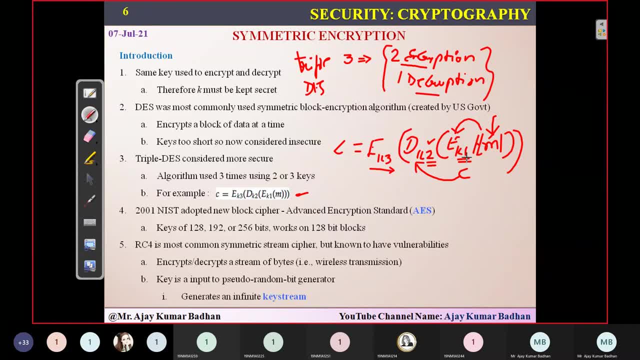 getting not the actual message, some other message, because i'm using the second key, not the first key. if i use the first key, then definitely i'll get this particular message, but i'm using a separate key here, so definitely you'll be getting another cipher, that is c2, and on that c2 you'll be. 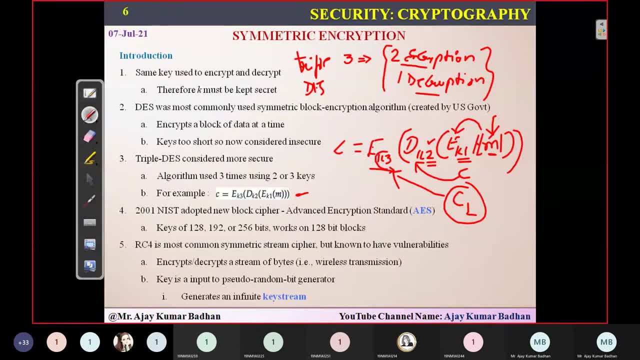 applying this particular ek3, that is, encryption using this particular k3. so finally, you'll be getting a cipher text, something called a c3, and this c3 will be transmitted to your destination. so it becomes very difficult for them to understand. means that, in between hackers, your man in the middle, attack. 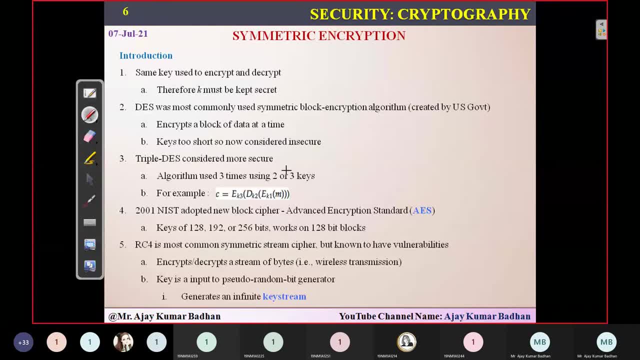 what we have seen in the previous session. they will not be able to know exactly what the message it consists of, because they don't have three different keys. earlier there used to be only single key. somehow they used to manage to get the particular key and they used to decrypt it. but now 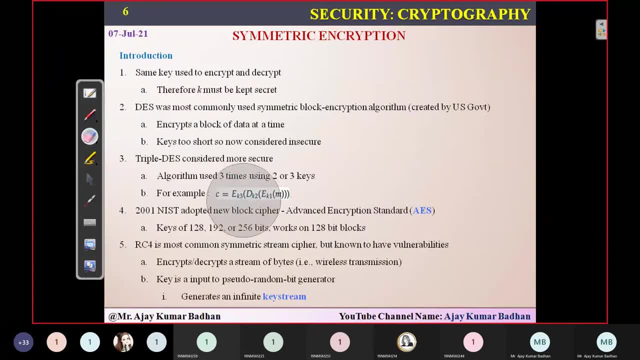 since you people are using three different keys here, definitely they mean they should have three different keys. then only they will be able to get the actual message and definitely they will not be able to be successful in getting that. so they will be not able to do that. but when they applied this triple des, what happened here is the 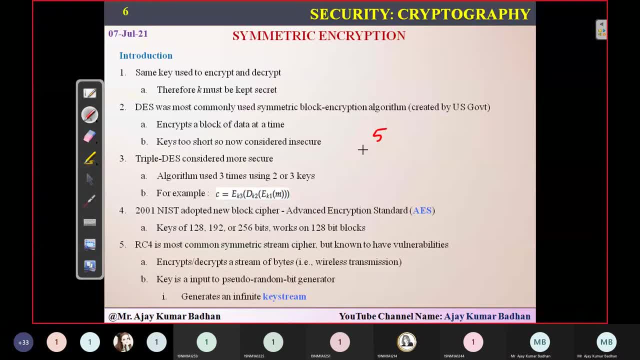 number of keys earlier. what is that? when single time you used to, we used to apply this particular ds means? or what is the size of this 56 between key? we used to use it right, but now this has been transmitted to 128, 192. so we have three different type of keys now. first time, 128-bit. next year. people can use 192-bit, then we can use 256-bit. and i'm telling you that when people are using 226-bit, then we can use 256-bit. and i'm telling you that when you're using two pcs, here you have more keys- number of keys. so now that's the given version. so now, once we've done this, we actually need another. 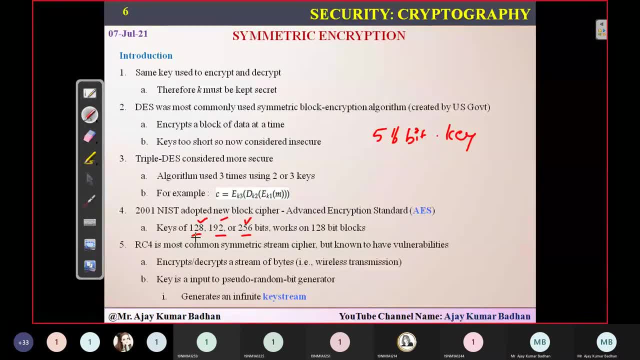 key. so i'm going to go to the next step, and that's the key s and that's the key. so i'm going to go to the. then we can use 256 bit and i'm telling you that when you are using such a higher c, where is 56? 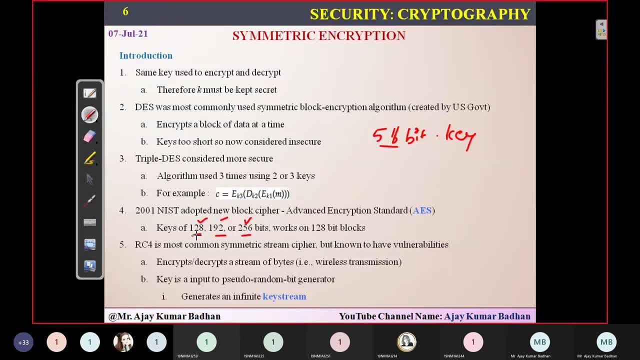 and where is 128? so when you use 128, it becomes very, very difficult for you people then what we call the system to detect, or the hackers to detect the actual output, and that's the reason. that is what i showed you in the beginning. now, how strong is your password? so what exactly you're doing? so? 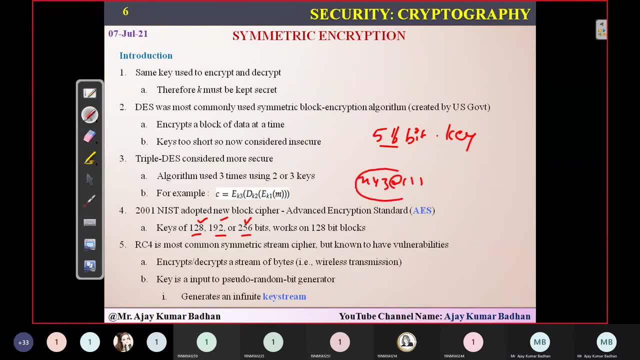 when you give a password, something like xyz, at the rate one, two, three for this, this will be applied. the ds algorithm will be applied, so it may be a 128 bit or it may be a 192 bit. so, based on that, what will happen? this xyz at the rate one, two, three will be converted into a different format. 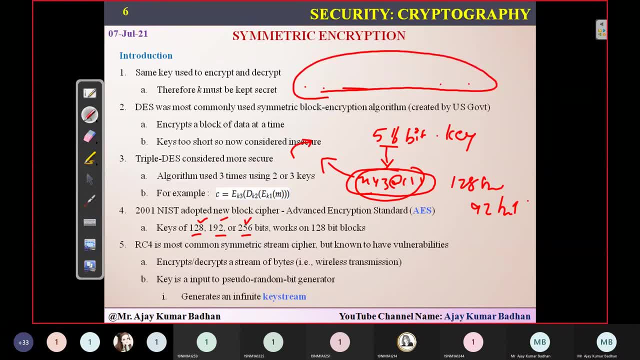 different format means it will be something very big message and this big message for a hacker to crack will take a lot, of, lot of time, and that you people have seen it right: some trillions of years, some billions of years. if you give only normal password, something like your phone number, your, 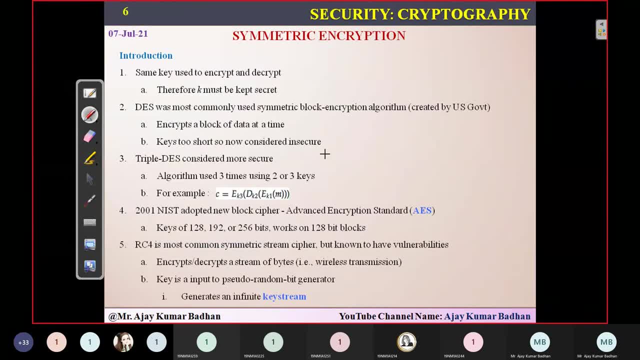 data, but it may take only 50 seconds to crack and it will be converted into a different format. and it will be converted into a different format and it will be converted into a different format or something like. you have already seen it right, so i'll tell you once again later on. whenever we have a free time, i'll tell you so. 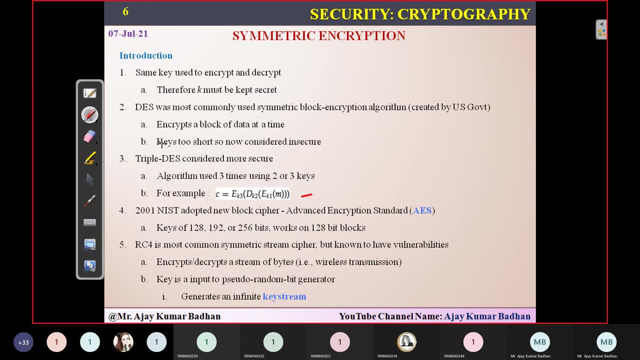 that if people can answer. so this is what comes under into this. so triple ds, you remember? so if you're applying ds for the only one time, so we are using a 56 bit key and whereas coming to a message we can use 64 bit message. but when you're applying triple ds, okay, triple ds advanced. 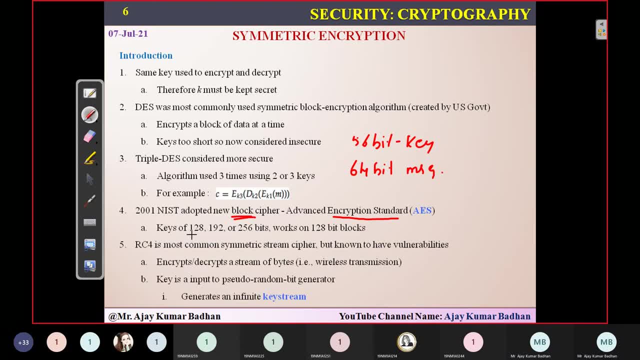 encryption standards when they have applied it. then what happened? the key size has been increased. not only key size, even the message size. earlier it is 64 bit, now they have increased it to 128 bit. and if you see the key size, the key size can be 128 bit, or it can be 192 bit, or it can be 256 bits. 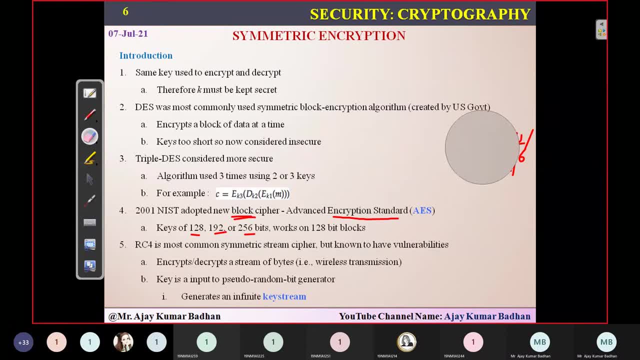 it's very, very difficult to crack the code. whatever the cipher text we are having, it's very difficult to crack it and get the actual message because of this particular case, and later on we had one more thing see, implementing this is also a very difficult thing to do because it's very difficult to crack. 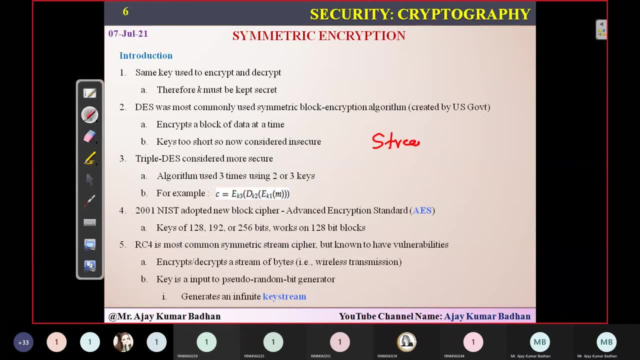 also typical thing, so definitely for that we have stream ciphers. then came to stream ciphers into picture. so what is stream? ciphers are nothing, but these are used to encrypt a stream of bytes, of bits, means, rather than taking a block like we, as i told you that we are using 64 bit. 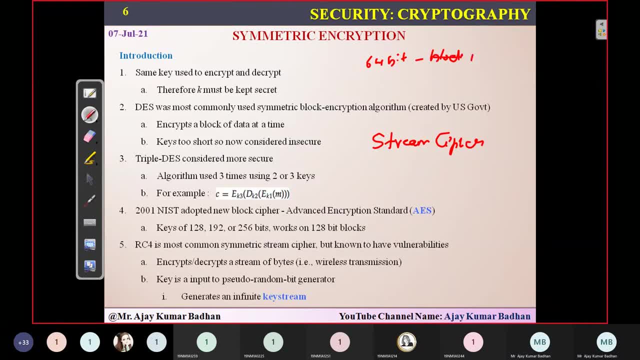 block means 64 bit message. that message is what we call it as a block suppose. let us suppose you are having a 25 bits, 128 bits message. so what happens here? uh, 64 bit will be taken first among this. uh, and that message will be. 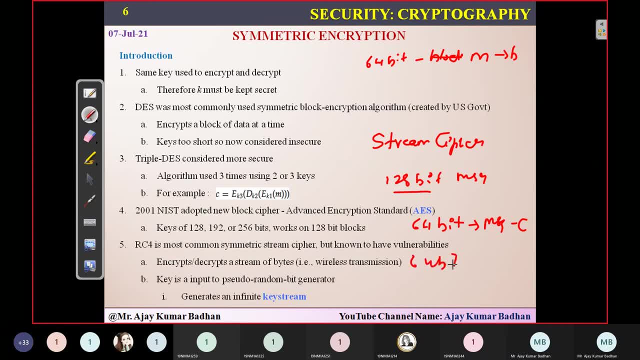 converted into ciphertext, then after that the remaining 64 bit will be taken and that message will be converted into ciphertext. what exactly you're doing? this 64 bit he is talking about as one block. so means if you are having a message of 128 bit message, this will be converted into. 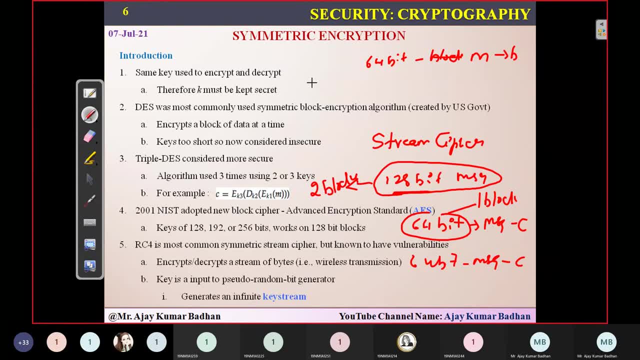 two blocks. okay, so the first block will consist of 64 bit and next 64 bit will be present in this particular. so this will be converted into ciphertext c1, this will be converted into ciphertext c2, and both this will be transmitted one after another, but what happens here? blocks means it becomes somewhat typical and implementing them is also. 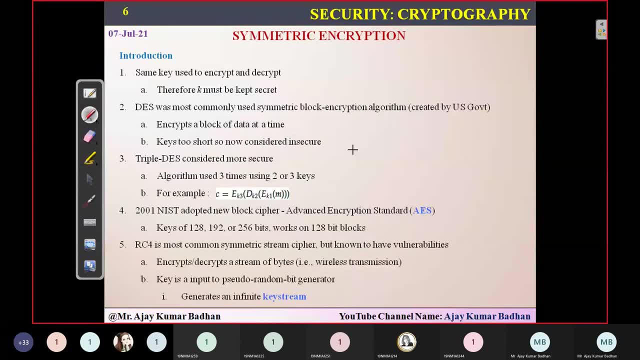 very, very tedious task. so, in order to overcome this, what they did is they came up with something called a stream ciphers- stream ciphers. what they do is, rather than taking the blocks- that is nothing but bits- they used to take bytes. they can use either bits or bytes, okay, and using these bits and bytes, they used to encrypt it. uh, and to 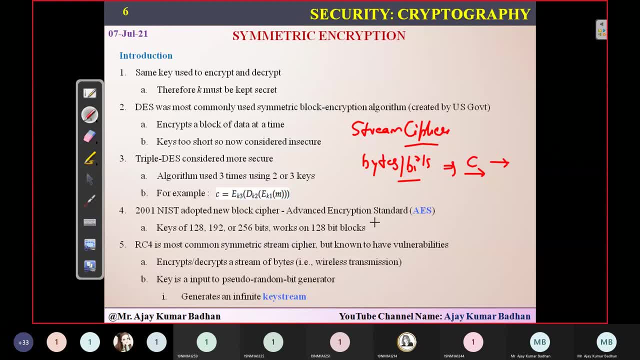 convert it. i mean, they used to convert that into ciphertext and transmit it. so for that, rc4 is one among them. rc4 is the most common stream cipher. what we use it- symmetric stream cipher- we use it okay. so here the. what exactly they are doing is they use something called a pseudo random generator. 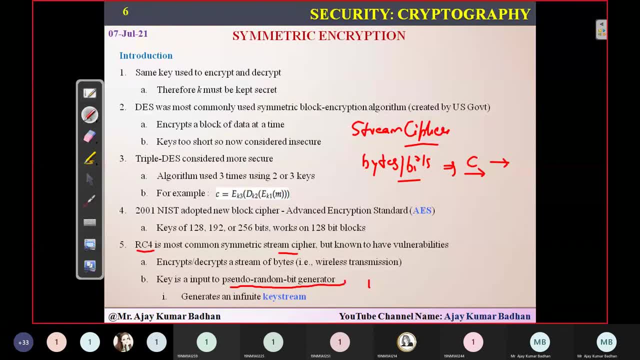 yeah, there is. this is represented. this is the one which is used. they use this particular technique, something like this, and then they use this particular technique, and then they use this particular something called a pseudo random bit generator. this is a generator. i mean, this is a kind of app. 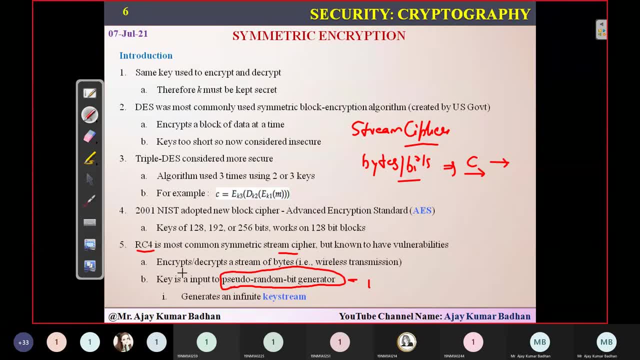 they used to use it and, within this, a key is given. whatever the key we are using, 56 bit or 128 bit or whatever it is that is given to this. now what this generator will do: he will be generating some stream of bits. he will be generating some stream of bits and that bits will be, like you know, infinite key. 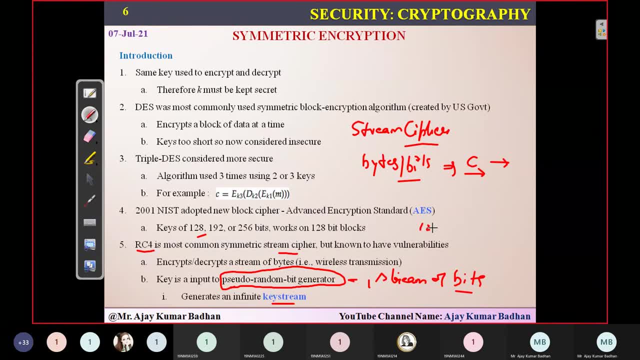 stream. we call it as it means very large. for example, if you are giving a 120, i mean uh, 256 bit will be converted into some 1026 bit size, so you can. you can see, 256 bit key is converted into 1026 bit key. that is very, very big. okay, so that is what is saying. generates an infinite key stream. 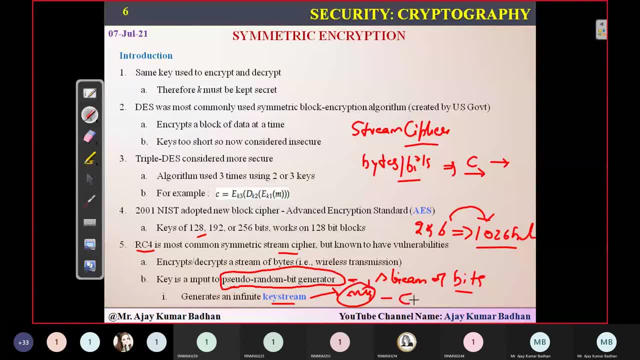 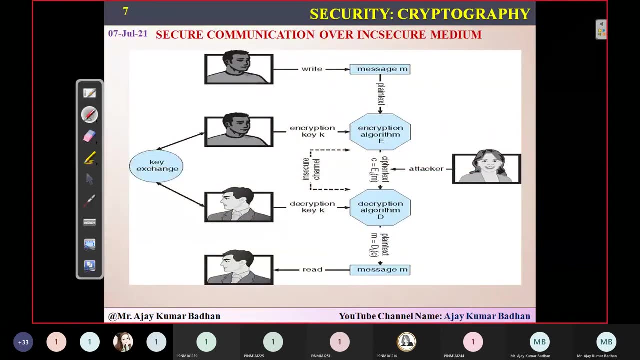 and this stream is applied to the message and then it is converted into a ciphertext and it is transmitted. so it becomes much more difficult for the hacker to overcome this particular thing. so this is what the diagrammatic representation in to do that. see here the user, this is a user and this is the same. i mean i mean sorry, this is the. 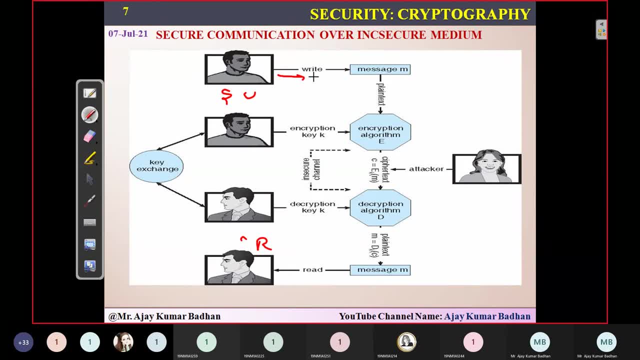 sender and this is the receiver now sender. what he did? he simply wrote a message here, normal m message. and what is this message here? we call it as a plain text message. normal message is nothing but plain text. nothing but people are writing hi. so this is a plain text message. that text message. 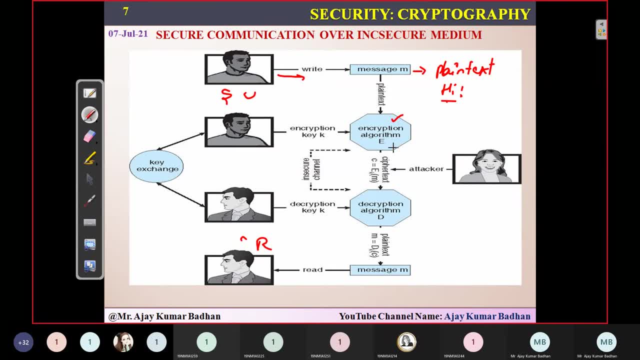 you people are giving to an encryption algorithm within your system, based upon the application you are using, and that encryption will be performed. how that encryption is performed. as i told you that there will be an encryption key, so this key will be given to this particular algorithm and 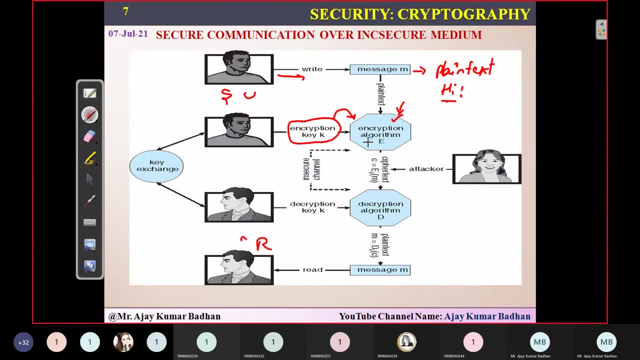 this. so you may be wondering, okay, sir, where exactly we are doing. well, this is done by your application. for example, if you're using whatsapp here and you're transmitting hi to your friend, so whatsapp will be performing this encryption. that's the reason we will not be seeing it. so what's up? what? 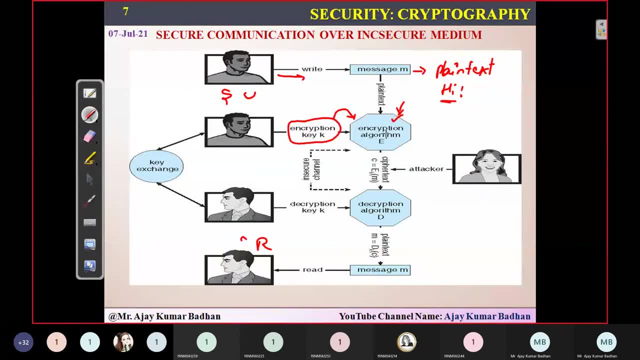 it will do, it will automatically encrypt. so whatsapp application consists of an encryption algorithm and key. what is the key here? and, as i told you, in between the sender and the user, between you and your friend, there is a code, histogram code. that code is what used as a key and that is what has been given to this particular 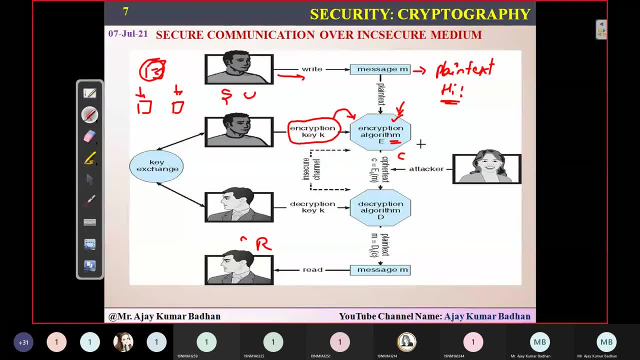 algorithm and this will be converting your normal plain text message into a cipher text and then it will be transmitted. now, if you see there is a attacker here- hacker or the cracker- he is trying to get so whenever he tried to hack the information. when you're transmitting over the 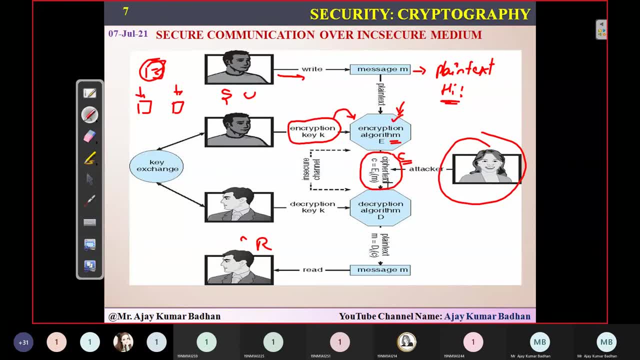 network. he will be receiving this message. what is the message here? cipher text, encoded message will be received, but this particular hacker will not have your key, this key, because this key is with respect to the sender as well as the receiver. this person will not have that key. so what is the message he will receive? is the encoded message and he will not be. 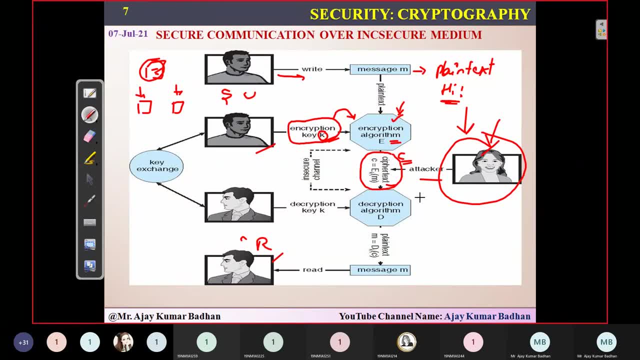 able to decode it. fine, that's no big deal. automatically, people can remove it up. so he will not be able to hack it up. so, finally, this message will be reaching to this person also. so what is the person here? receiver: he will be having the key. now, that key, he will give it, so, in 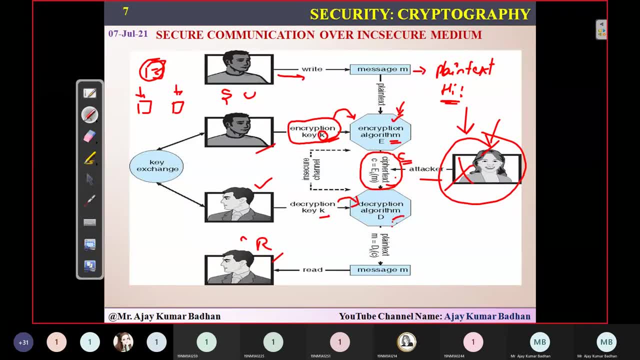 this particular case, the receiver is sending a message, so what will happen is here. so the whatsapp application of this particular receiver will be performing decryption and finally a plain text message will come and this message will be read by you people, so you will be ultimately getting a message high. now what happens here is you will be transmitting a message. right, you got. 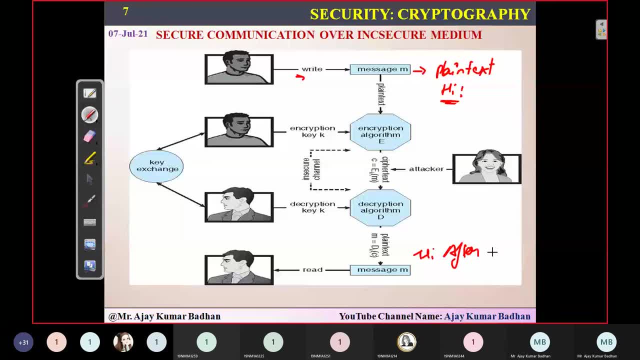 a high here. so definitely you'll be responding something like: hi, after a long time, after a long time, you're transmitting now what happens here. so this particular receiver, whatever the receiver is, the message he is sending here now, here, the same key is user to convert this into a cipher text. 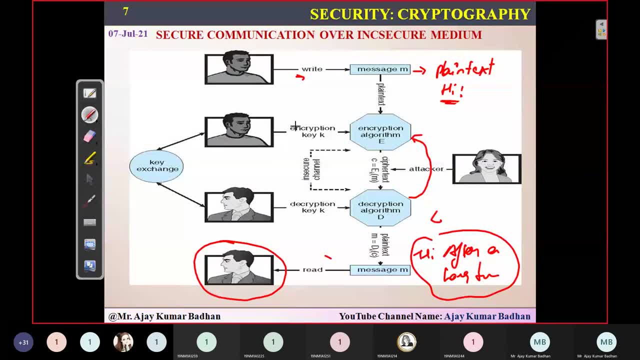 and that cipher text will be transmitted here. same way, this sender will be giving a key, that cipher text message will be again converted into a plain message and this particular plain message will be read by this particular sender. remember, okay, so when this person is sending earlier, what 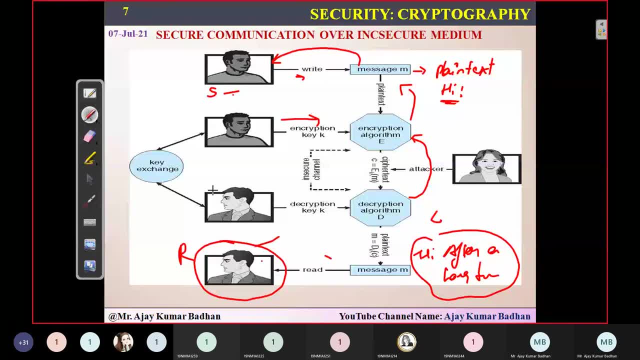 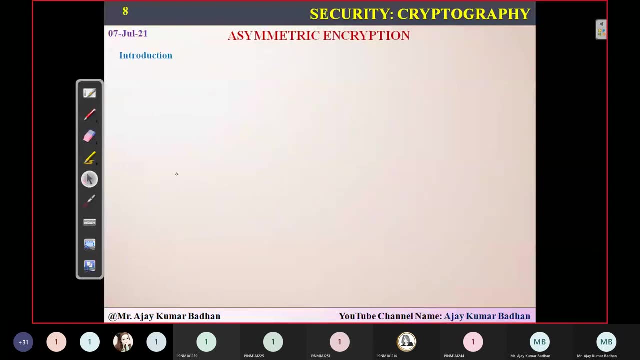 did. i say: he is the sender, he is the receiver, but when he is sending the message, he becomes the sender and this becomes a receiver. this is a vice versa kind of a format, what we are representing here. okay, so i hope you people are getting it so okay, fine, so we'll stop here in the 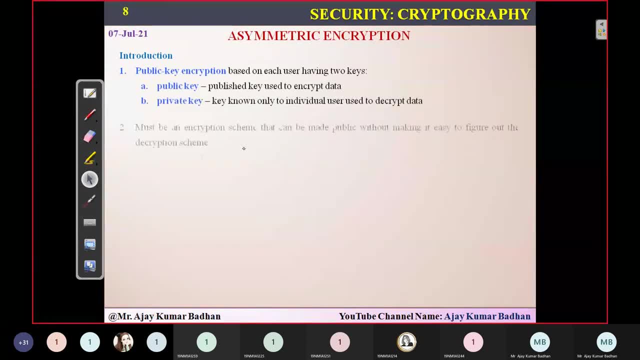 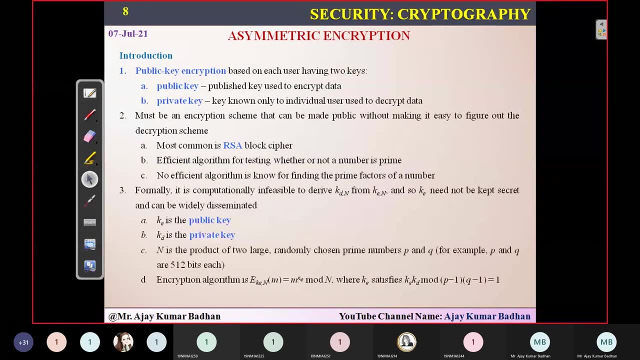 next session we'll be discussing about asymmetric. this is something important and on this we'll be working some problems also, so that people get something- no more benefit related to this- people can understand: yeah, this is a formula we are having here. you can see, these are the formulas we 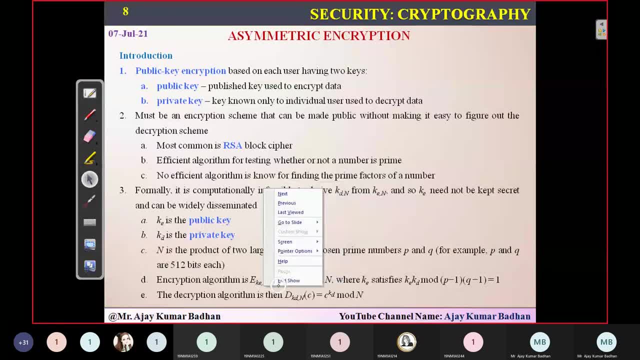 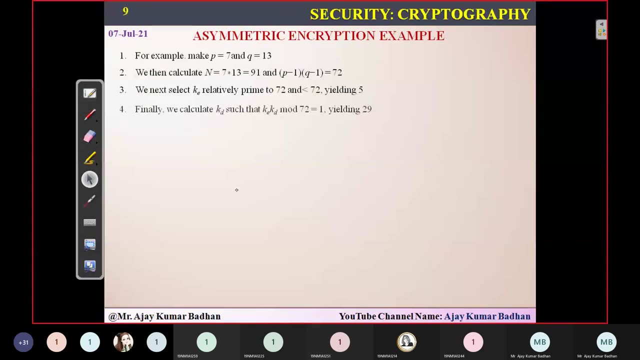 have, so you can see these. these are the formulas. uh, what we are exactly using here? this one. so i will explain in the next session and we'll be doing some problems with respect to that. these are very easy and interesting. yeah, there is example also here here. this example will discuss.